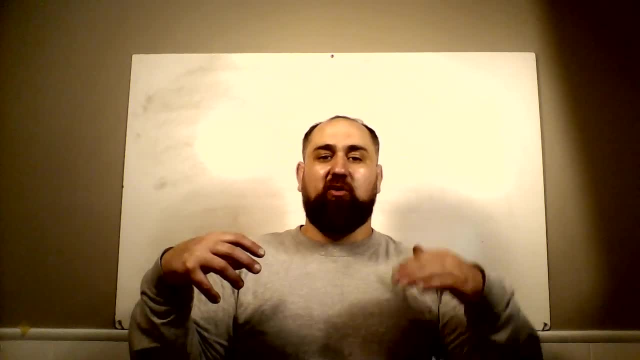 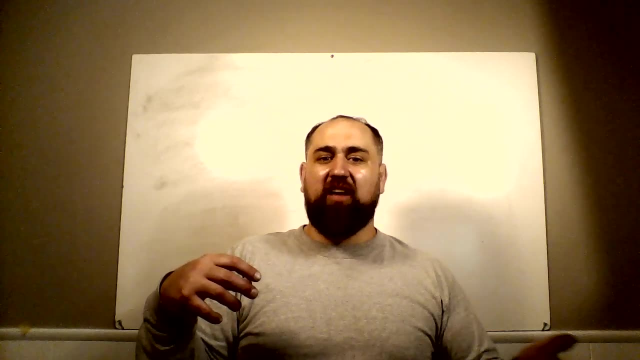 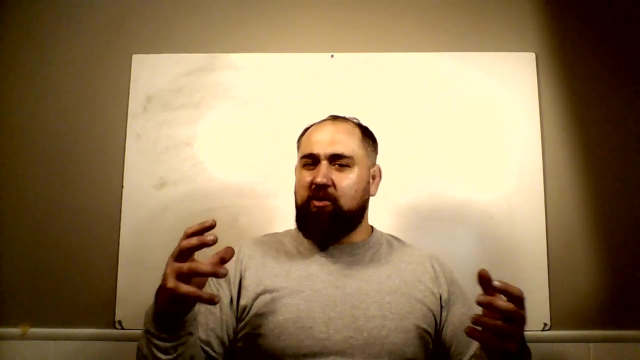 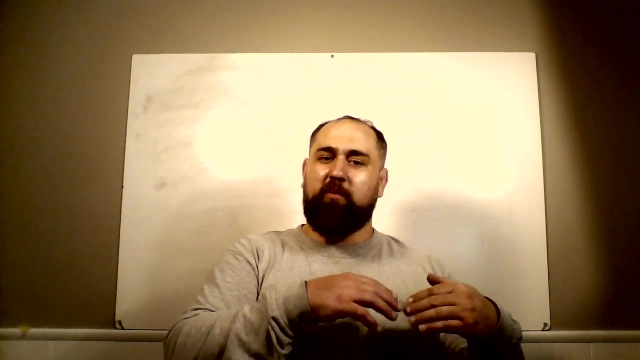 that allows you to maximize or minimize a quantity like energy, velocity, distance. It's very similar. just instead of taking a derivative and setting it equal to zero to find the maximum and minimum, you're going to be going through another process that's going to allow you to pull out the maximum. 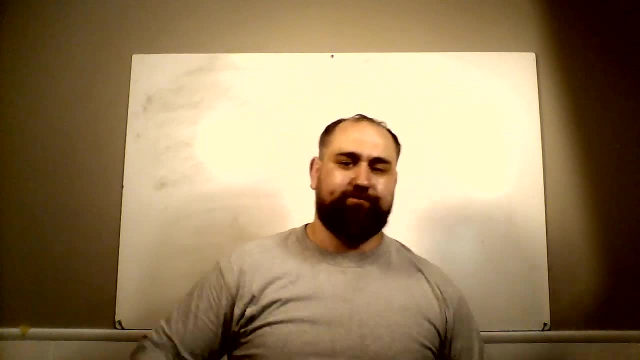 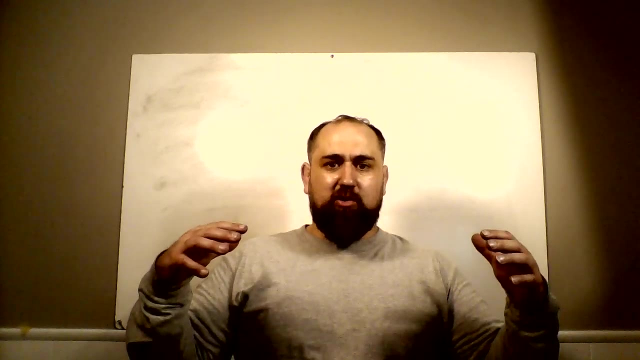 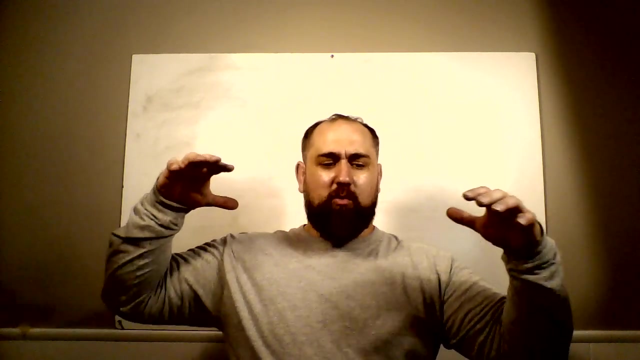 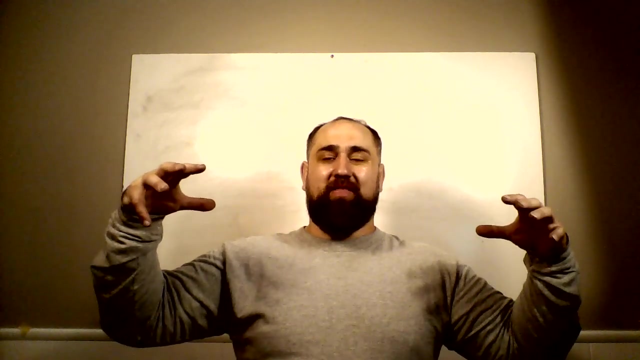 or the minimum function itself. Part of what we're going to go through is we're going to look at not only one-dimensional situations, but multidimensional. We're going to have functions that are multidimensional and we're going to have to pull out the one solution that is going to maximize or minimize a quantity. 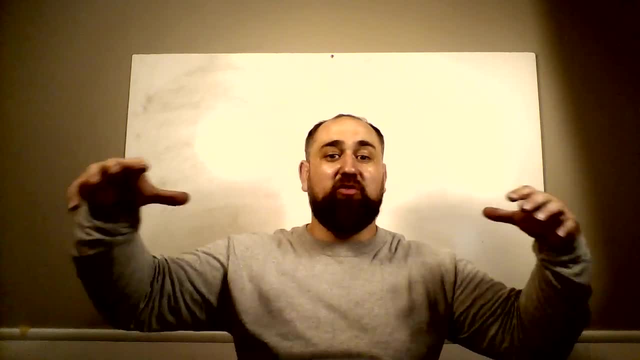 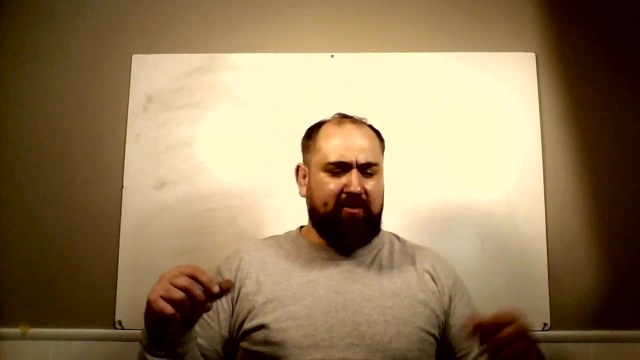 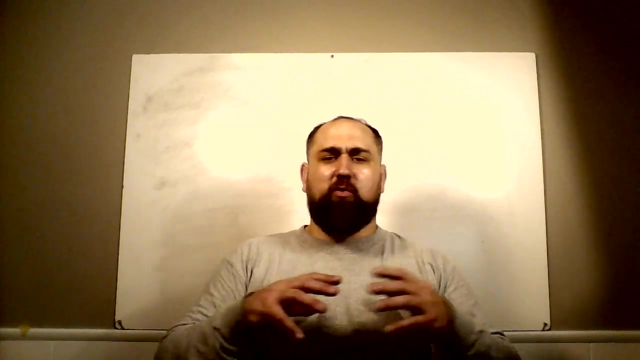 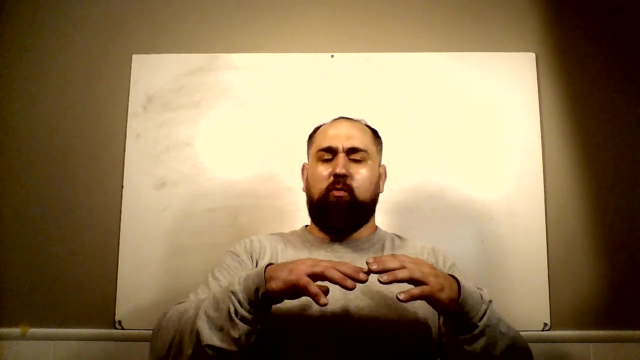 and we're going to have to pull out the one solution that is going to maximize or minimize a quantity over this multidimensional space. We'll also take a look at dealing with boundary conditions. For example, if we were designing a bridge, the bridge we would maybe design it to be optimally shaped for strength. 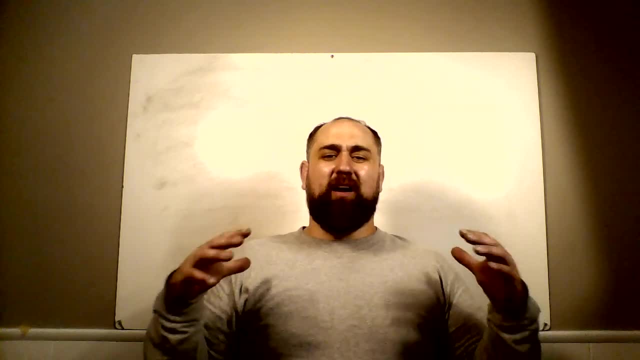 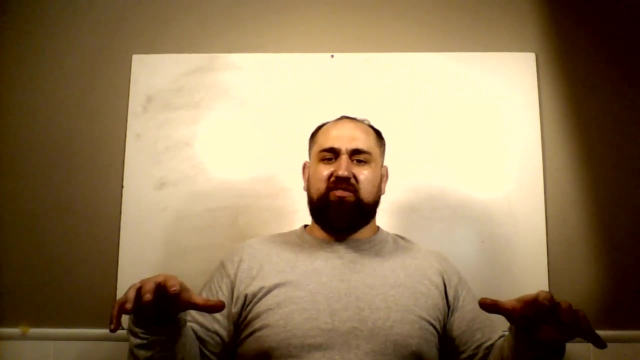 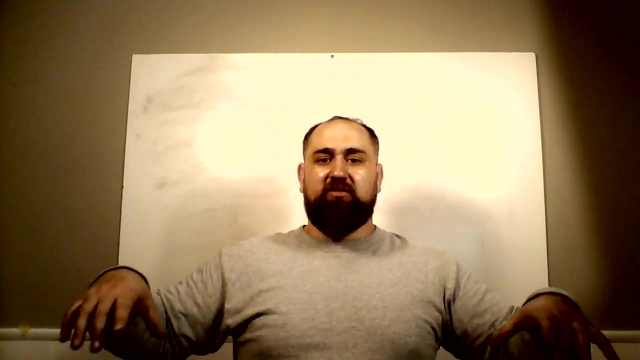 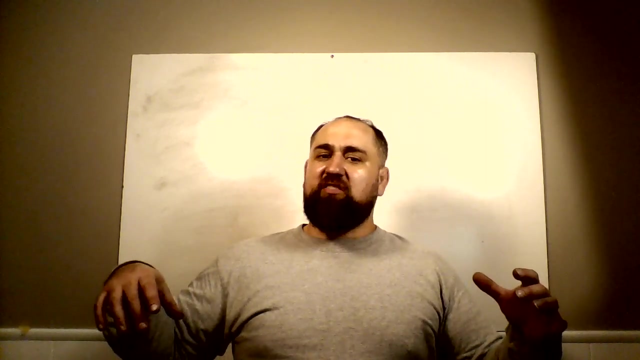 We'd want to pull out that one function that optimized strength- Typically the boundary conditions would be a given. It has to land on the ground right here, so our bridge has to go from here to here. In other applications there won't necessarily be a specific endpoint. 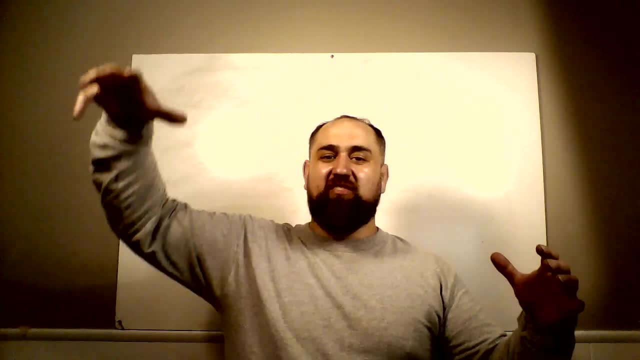 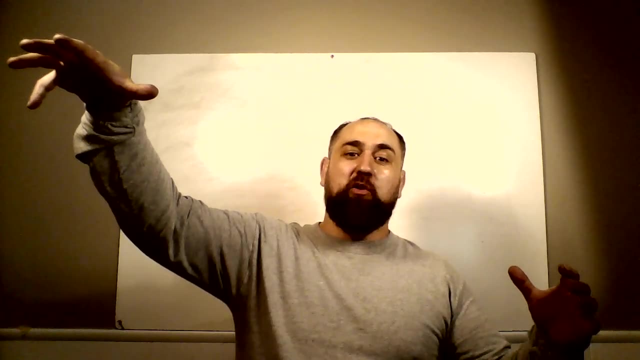 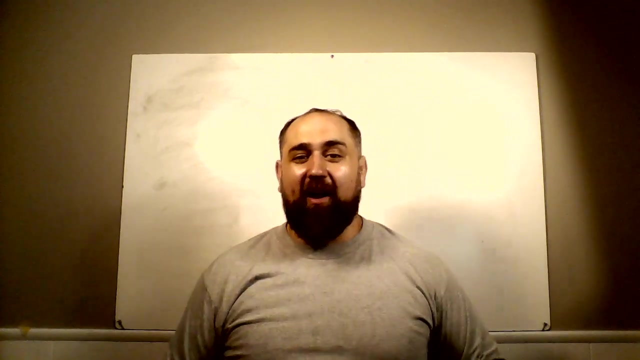 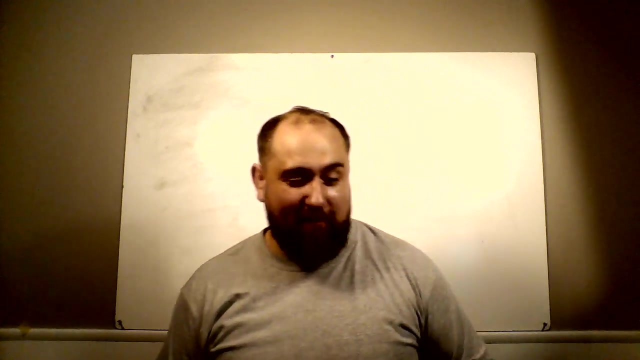 We'll allow those boundary conditions to vary so that we can determine the optimal boundary condition as well to further minimize the desired quantity. It's an unbelievable type of mathematics. I just can't wait to get into it. Anyways, on this first video, 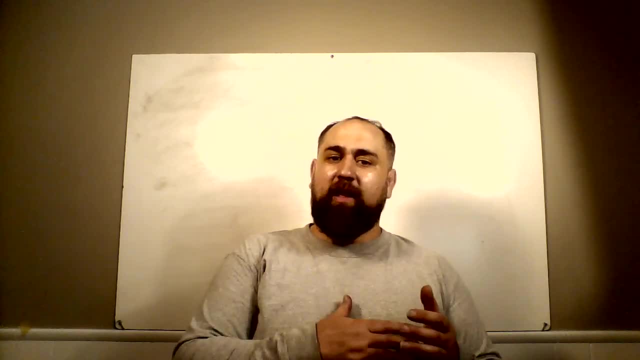 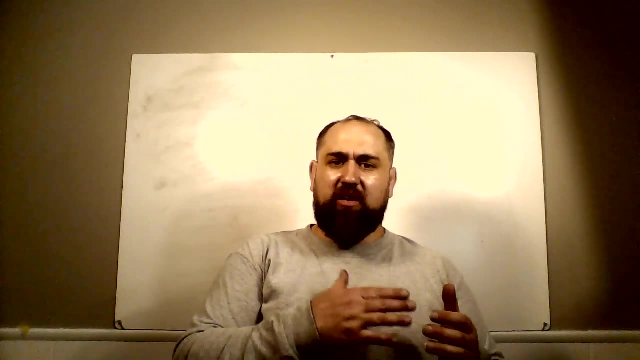 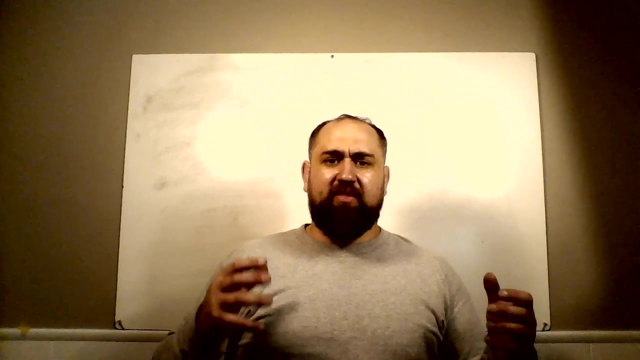 we're going to focus on deriving the equation that is the foundation of calculus of variations. It's what we're going to use over and, over and over again in solving these calculus of variations type problems. That's called the Euler-Lagrange equation. 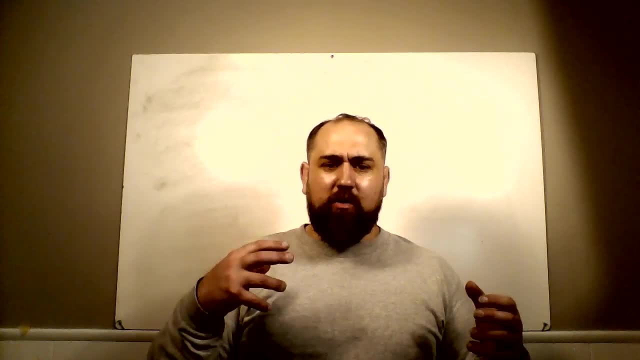 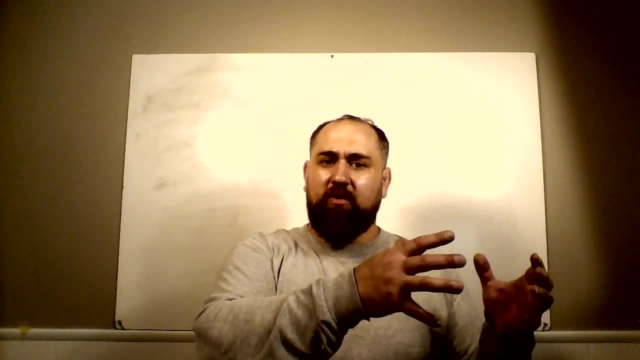 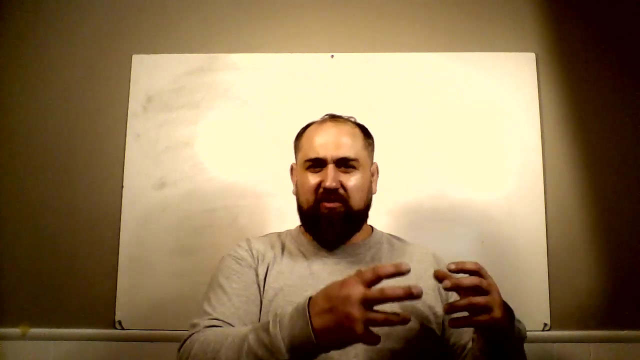 While we're deriving this Euler-Lagrange equation kind of simultaneously, we're not going to solve a calculus of variations problem, but we're going to set it up That way you can kind of get a feel for the types of problems that you can solve. 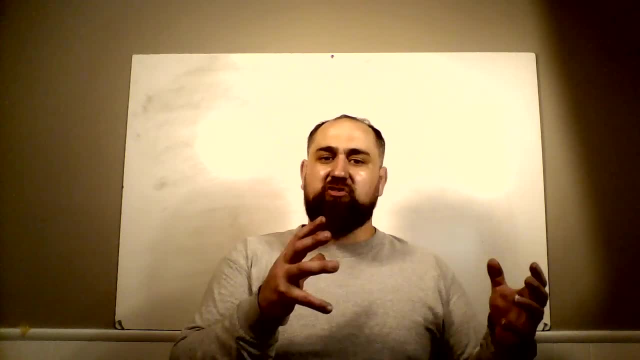 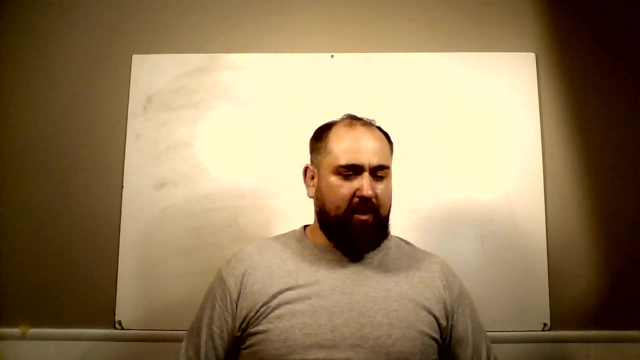 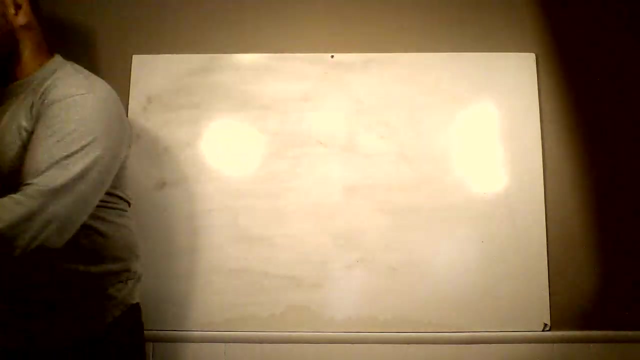 and the general structure of calculus of variations. This first problem is called the Brachistochrome. Let's start setting it up here. So what we're going to do is we're going to start with the Euler-Lagrange equation, With the Brachistochrome. 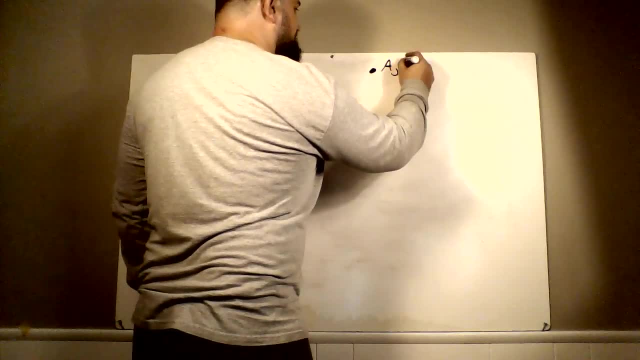 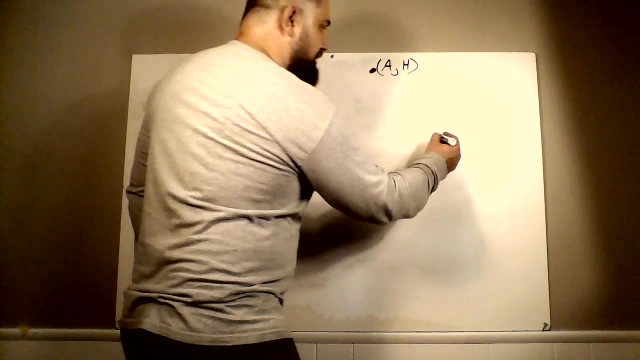 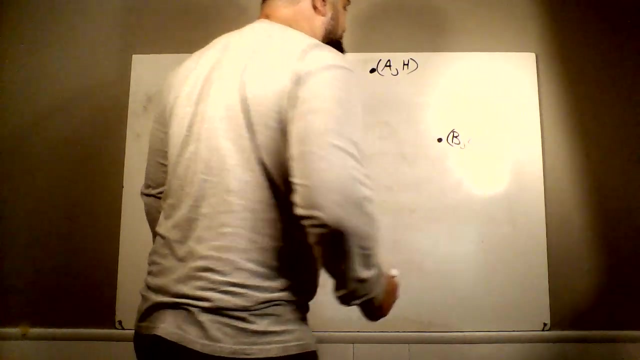 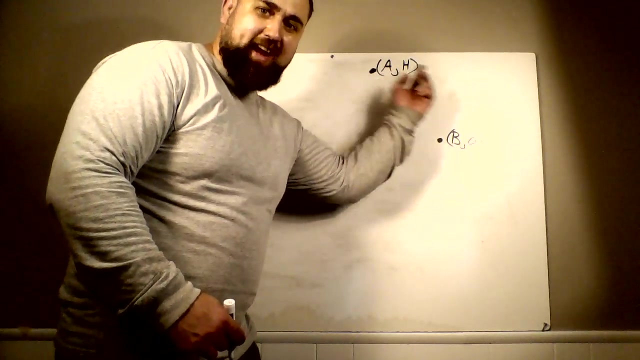 we have two points in space. The first one we'll say is A-H, X-Y, A-H, And then the second one is B-0.. Okay, And A is not directly over B, so they're staggered And we want to connect these two points. 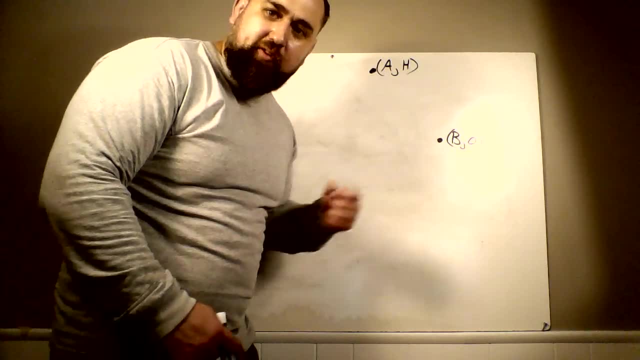 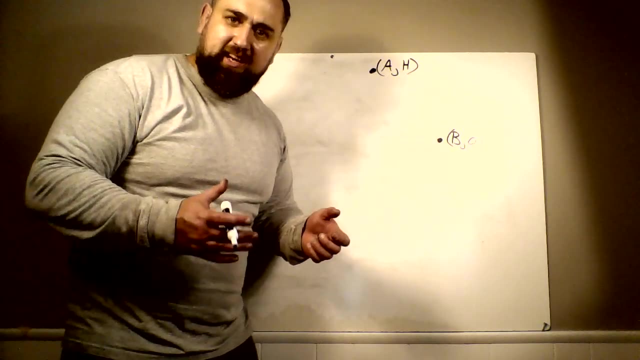 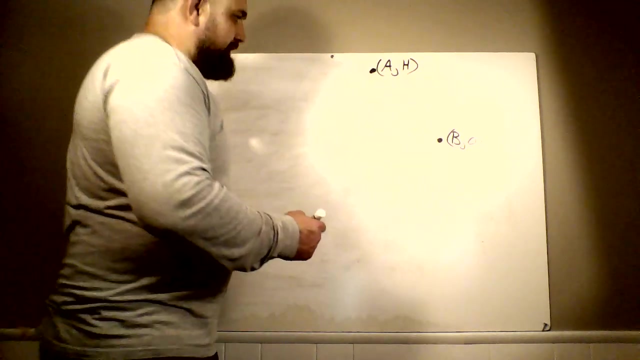 such that we want to connect them with a frictionless roller coaster, such that the time of travel under the influence of gravity alone is minimized. Okay, So we want to minimize time. Now we could connect them with a straight line, And that minimizes distance. 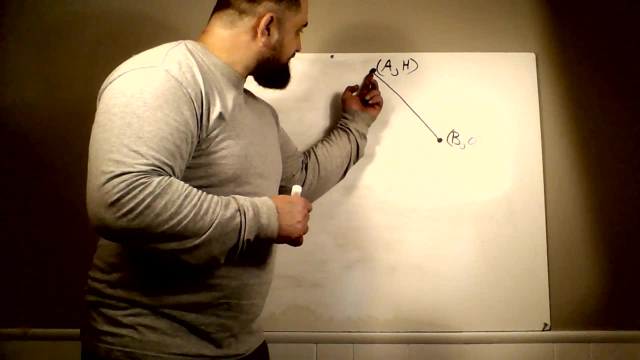 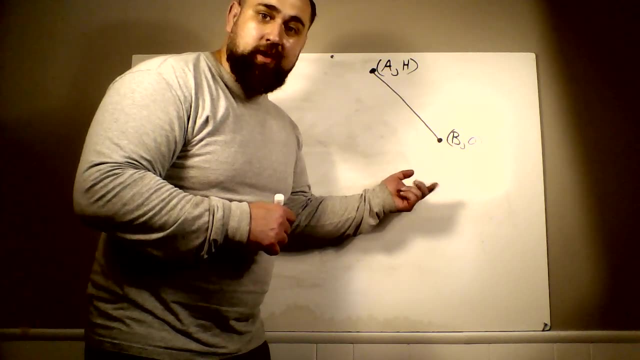 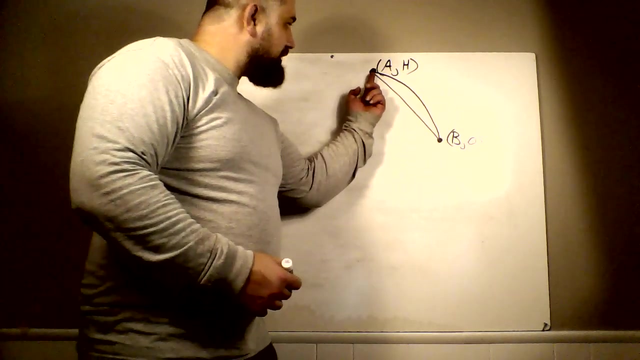 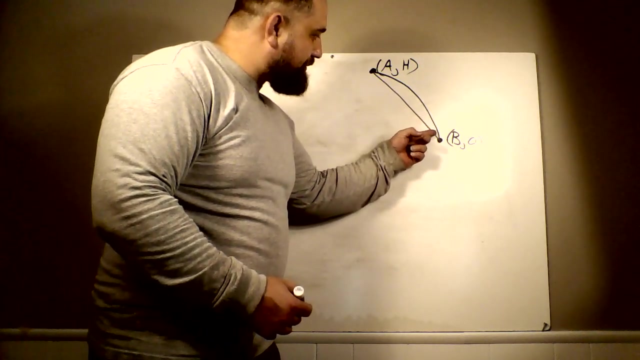 But we can't guarantee that there is enough acceleration to guarantee that time is minimized. Okay, We can do something like this, where we have a little bit longer distance but we have a greater acceleration at the bottom, But intuitively we have a. 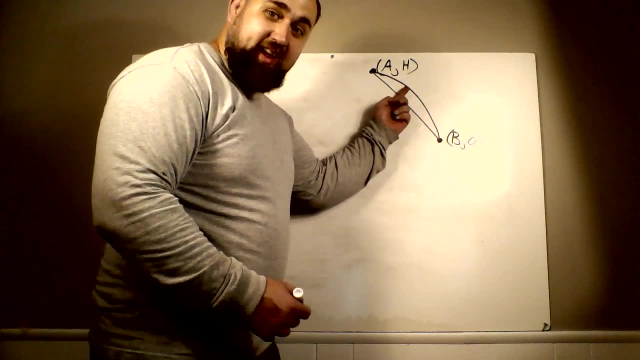 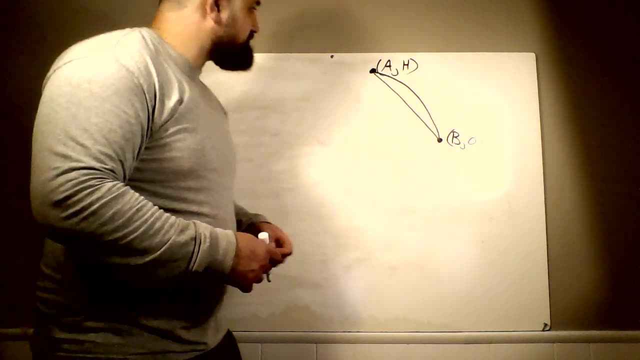 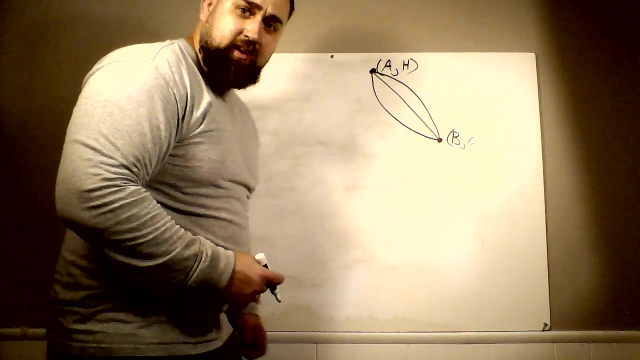 much slower acceleration at the top, And so it's going to turn out that this is not going to be our optimal solution. Okay, We can look at the kind of opposite of that, Something like this: Now, intuitively, this is a longer distance. 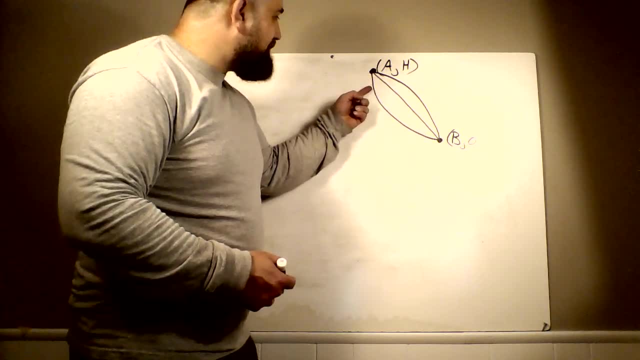 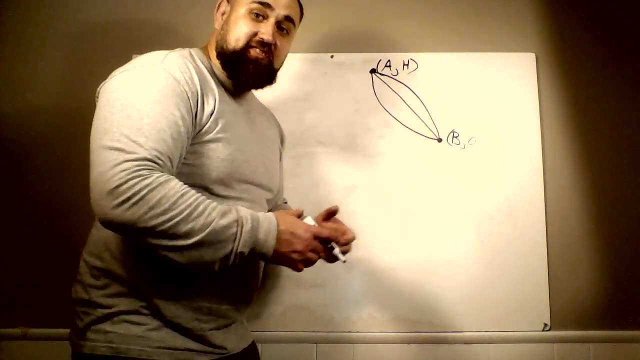 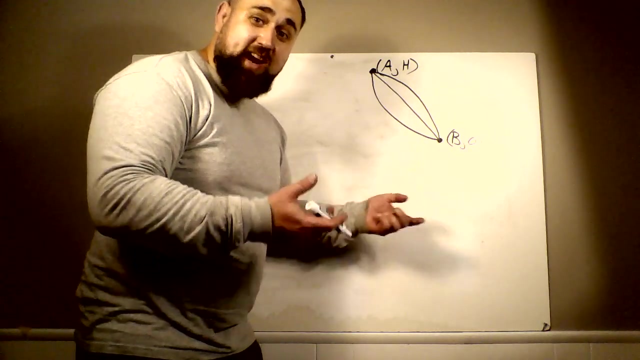 than the straight line, but we get a much, much greater acceleration initially, such that our average velocity is sufficient to account for the additional distance traveled over the straight line. So it turns out that our curve is actually going to be something like this: 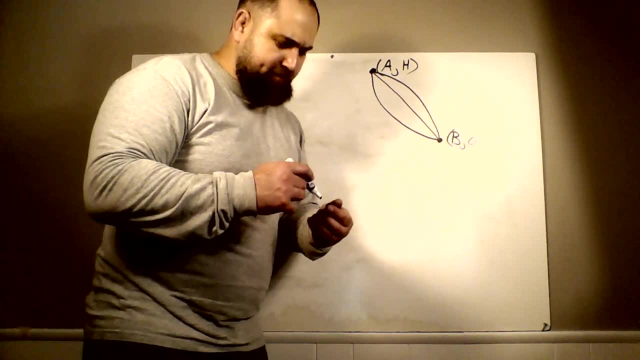 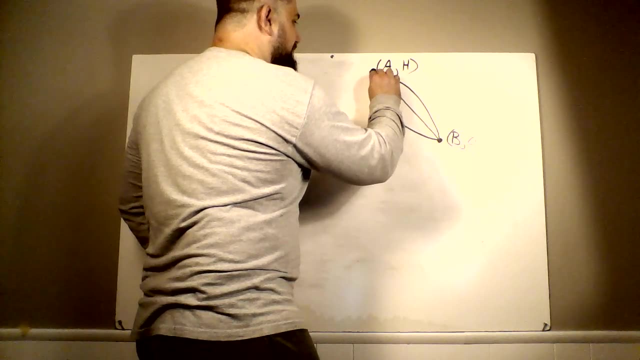 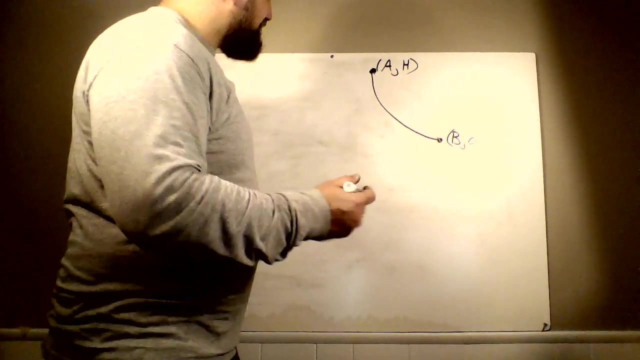 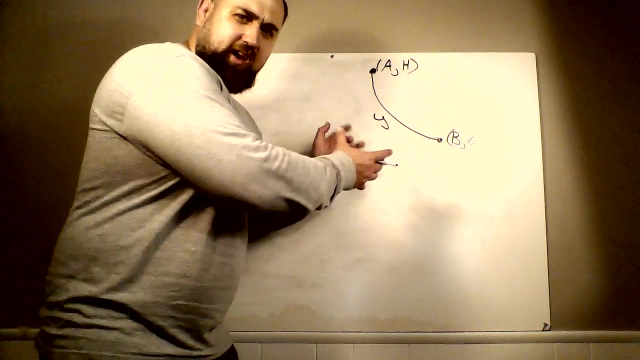 So let's go ahead and start setting up some of the equations so we can see why We will need to set up a little bit of nomenclature for this. So we're going to designate the optimal solution, y. Now we're not assuming the solution. 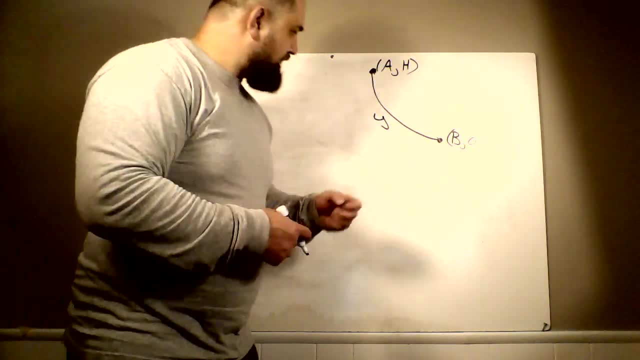 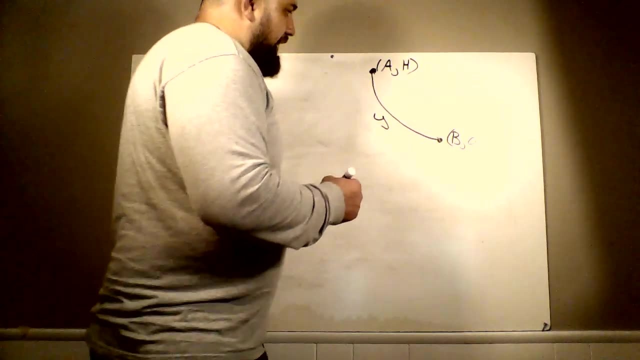 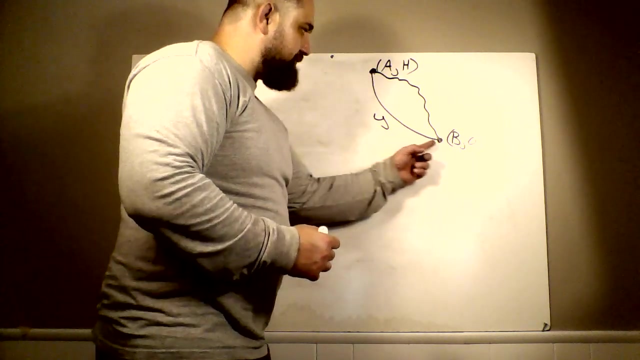 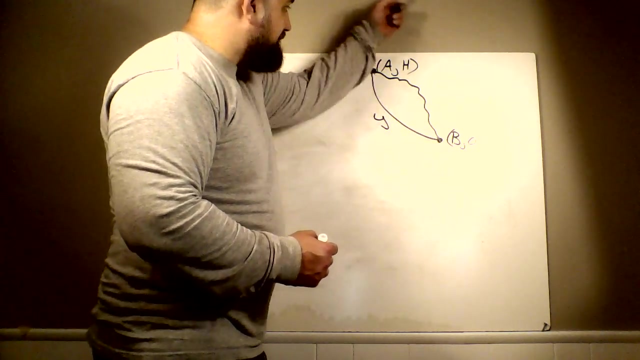 We're just picking something as the solution y, We don't even know what the function is, And then we're going to analyze a variation off of the ideal curve y. So there are infinitely many variations because there are infinitely many ways to connect a and b. 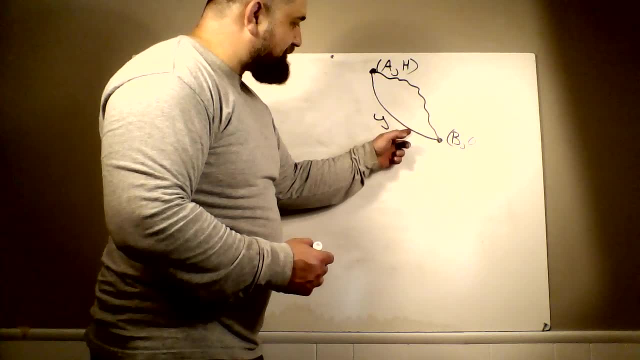 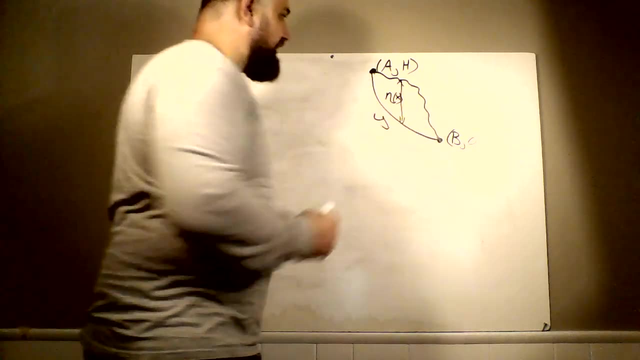 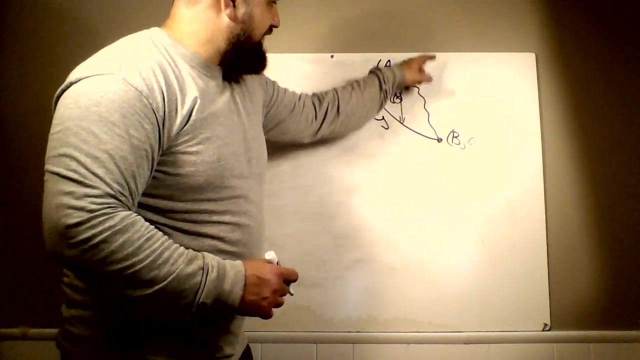 And so we're going to designate the difference between the optimal solution and the variation as being eta of x. It's just a function of x. Okay, so we have our optimal solution and then any variation. the difference between the optimal and the variation is: 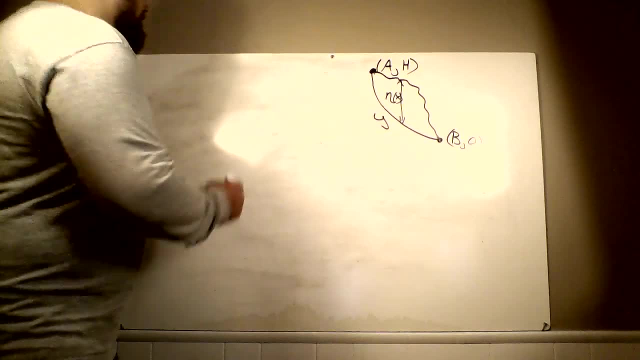 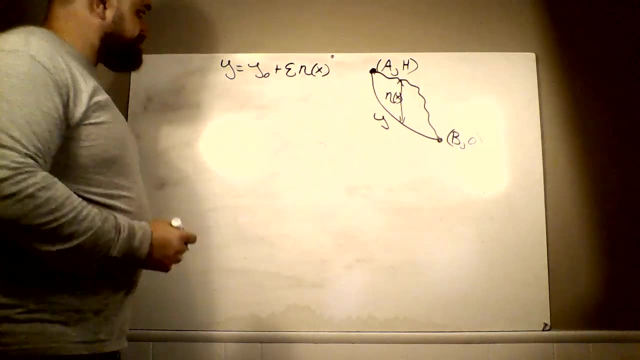 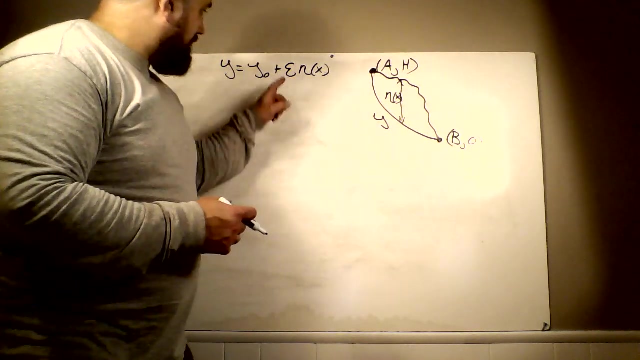 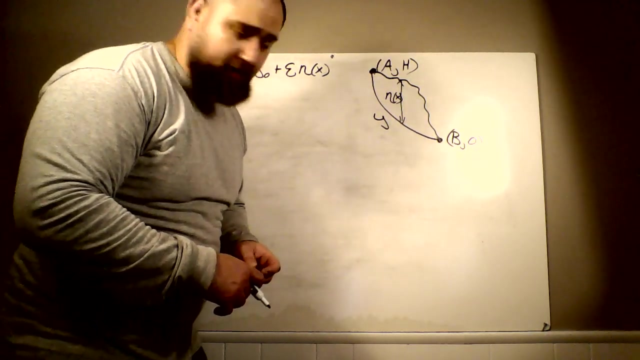 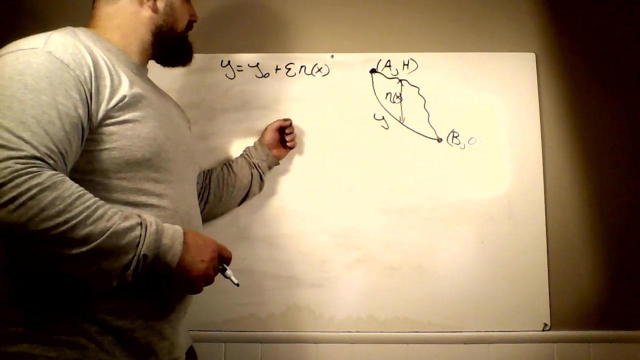 eta. Okay, we're going to say that epsilon is a function of sorry, is not a function of x. So with respect to x, epsilon is a constant. Okay, so when the variation is zero, we have y is equal to y. 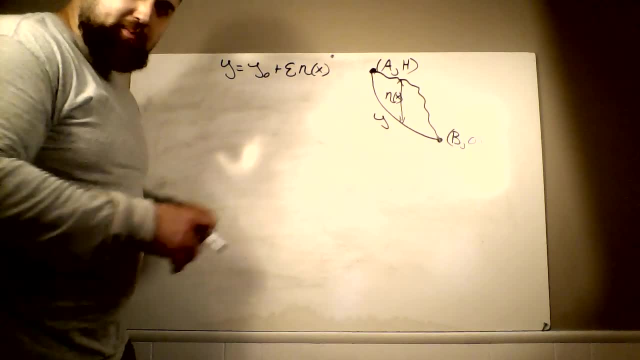 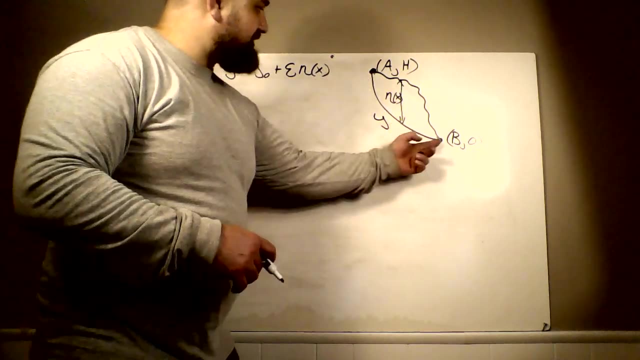 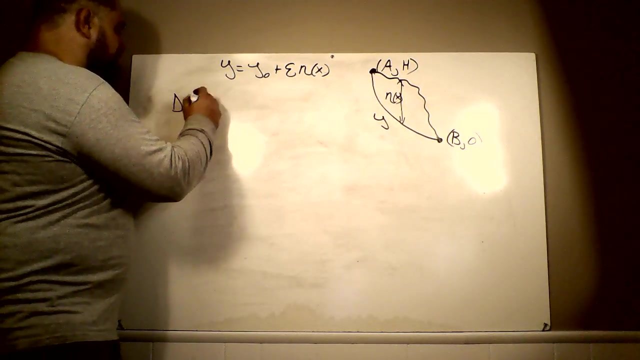 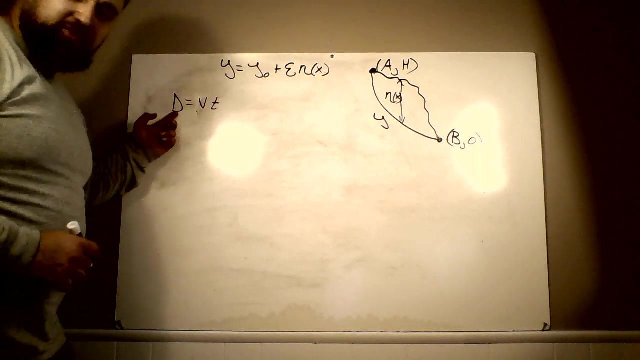 not. Okay, let's kind of skip over that for a second here and let's get into analyzing this. We have a distance equals rate times, time type problem. So from algebra we just have velocity times. time is equal to the distance. Okay, since 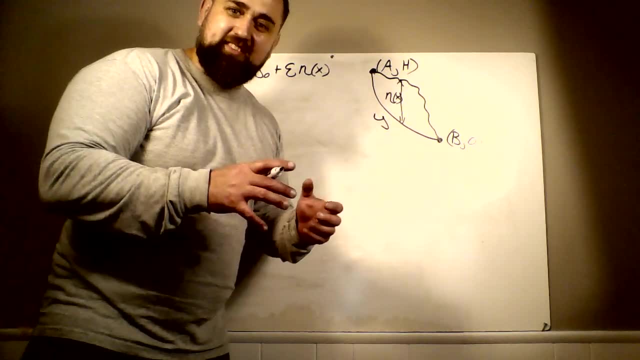 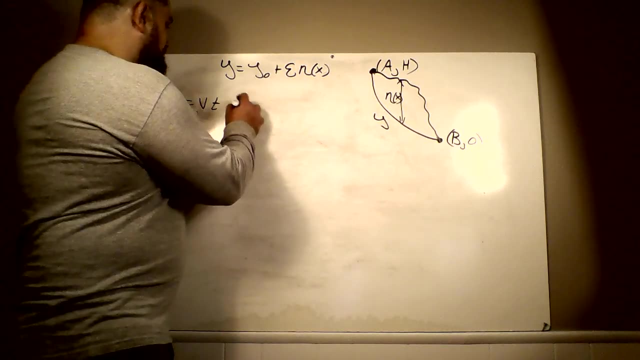 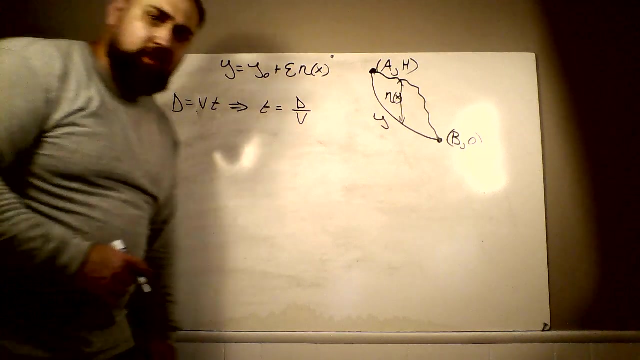 we are trying to derive the function that minimizes time. we want to go ahead and solve this for time. That's what we're going to be minimizing. So t is equal to distance divided by velocity. Now we can't directly apply this to this equation. 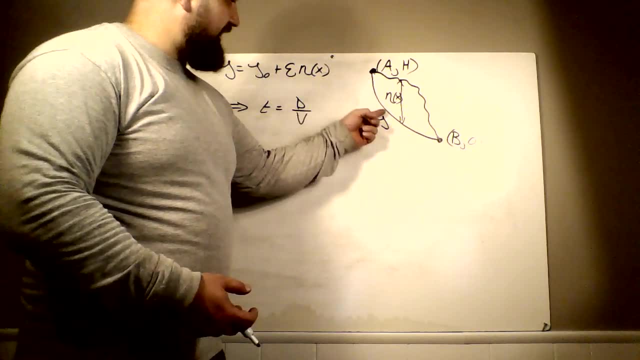 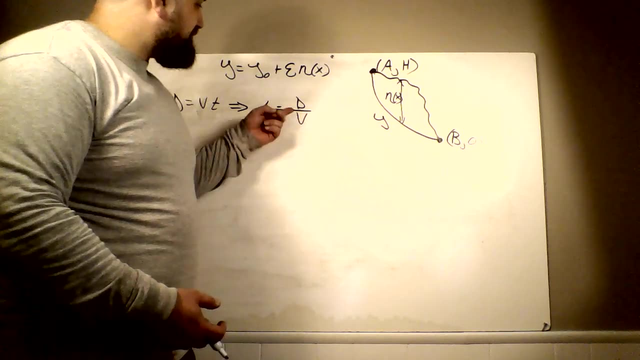 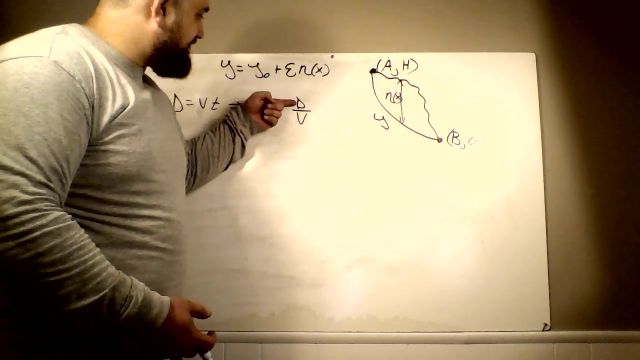 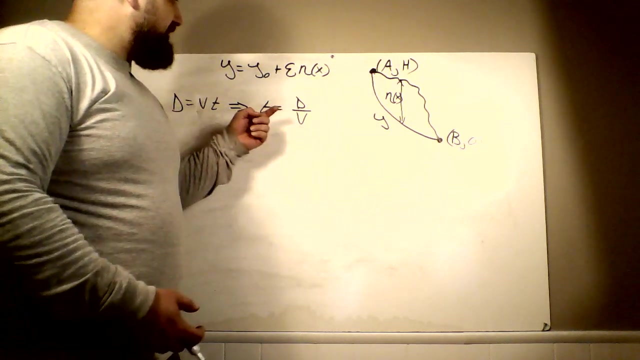 because the velocity changes as you fall, And so what we have to do is we have to put this into differential form, and then we analyze the distance over velocity, over each infinitesimal arc length, and then we add up those infinitesimal times to get the total. 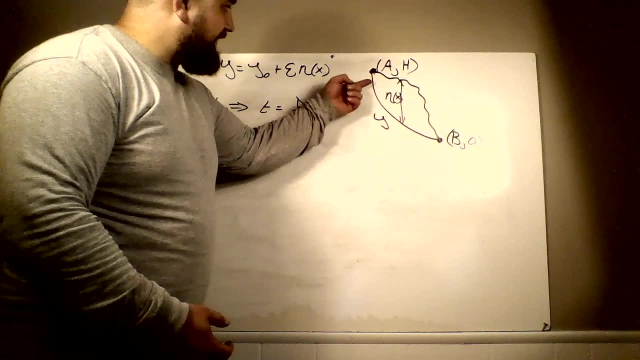 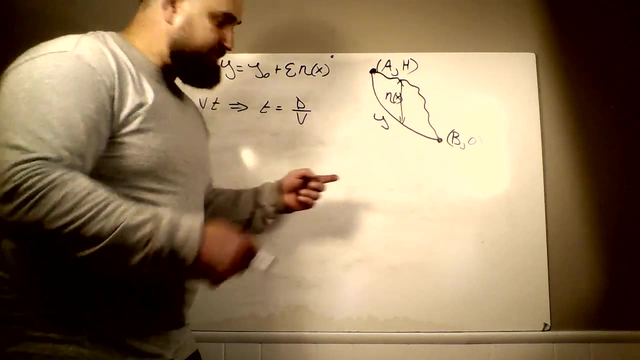 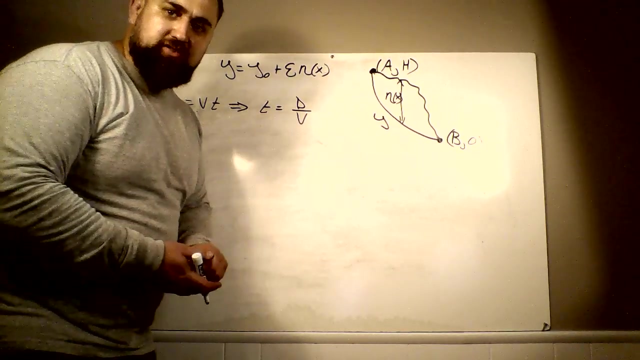 time. So we're going to analyze the infinitesimal times, in essence over the entire arc length, We're going to sum them up And then that gives us the total time. Okay, so we'll start by writing d in differential form To do that. 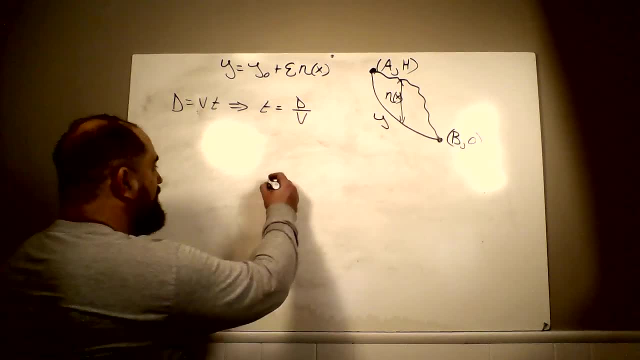 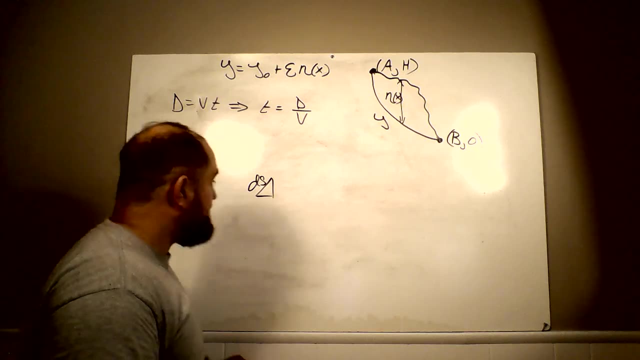 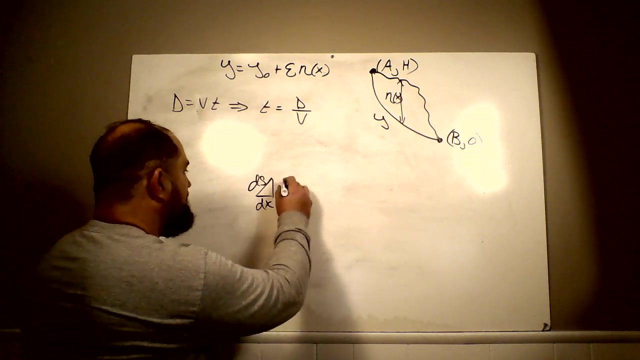 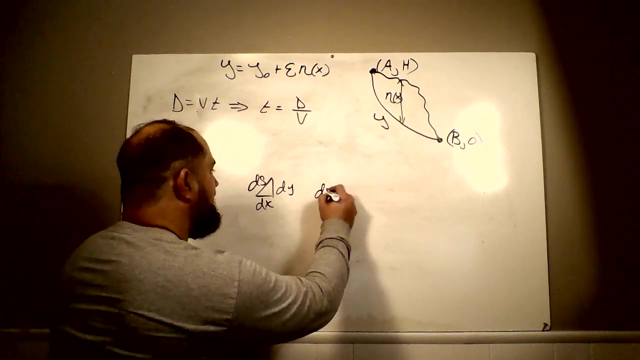 we use multivariable calculus. We remember that we have the hypotenuse of the differential. rectangle is sorry, triangle is dn. Then we have dx dy. Applying the Pythagorean theorem, we just get: ds squared is equal to dx squared. 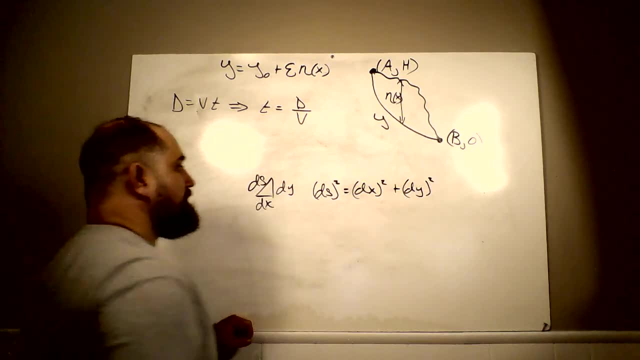 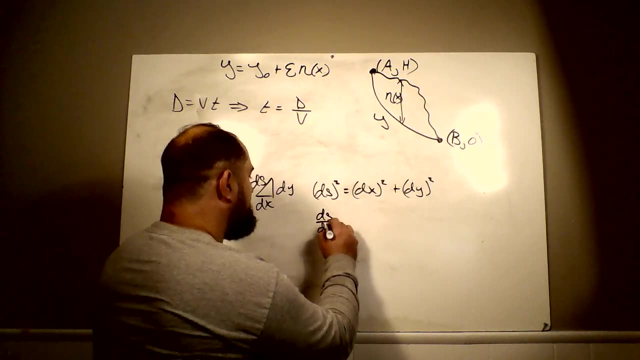 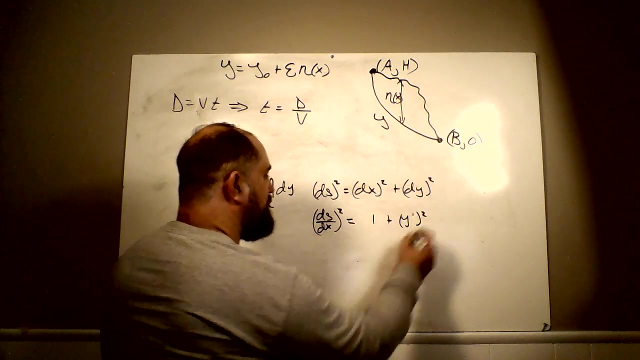 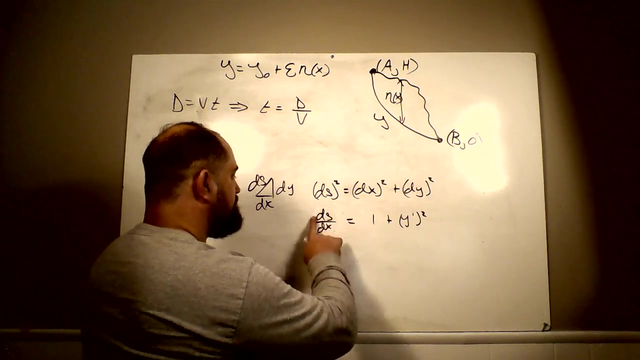 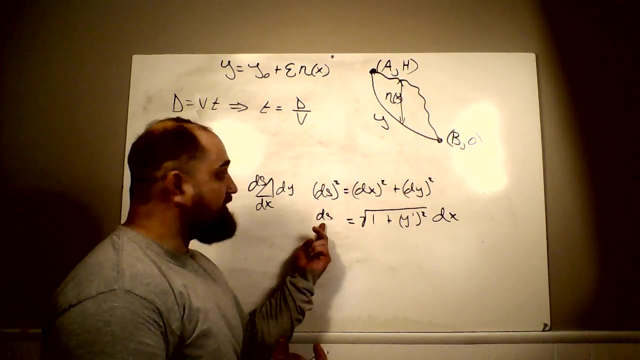 plus dy squared. Dividing by dx squared gives us ds over dx squared is equal to 1 plus y prime squared. Now we take the square root and then we multiply by dx, So our infinitesimal arc length, our d, becomes our infinitesimal arc length, dx. 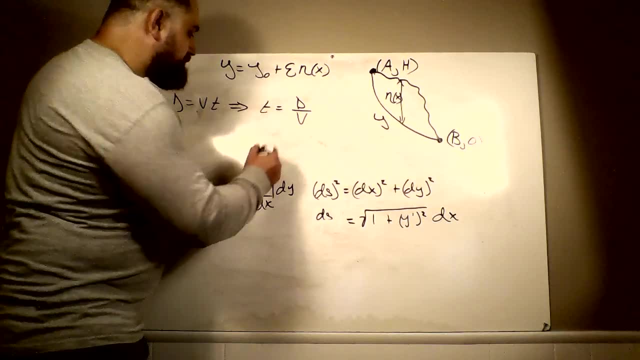 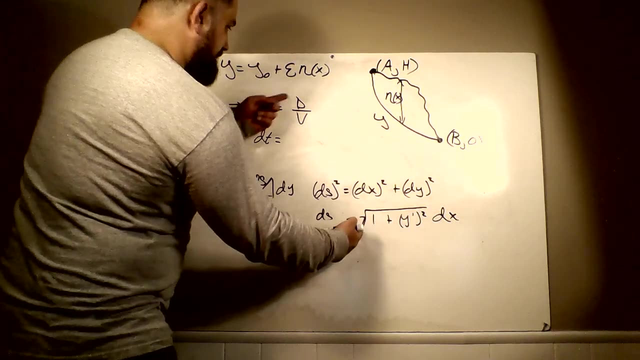 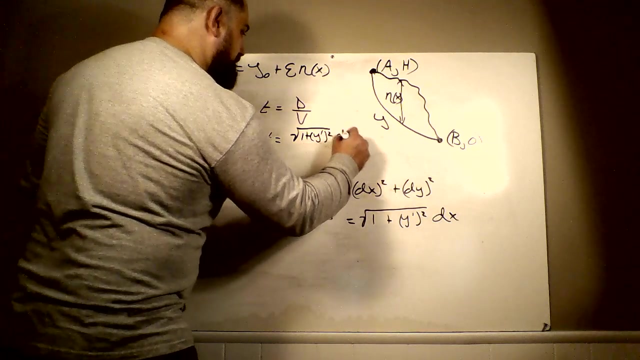 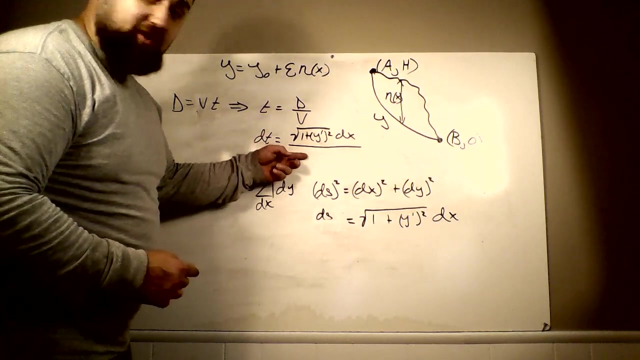 Which is this. So we're going to write dt is equal to this is our d. what we replace our d with 1 plus y, prime squared dx, And then we need to do a similar type process to write v into differential form. 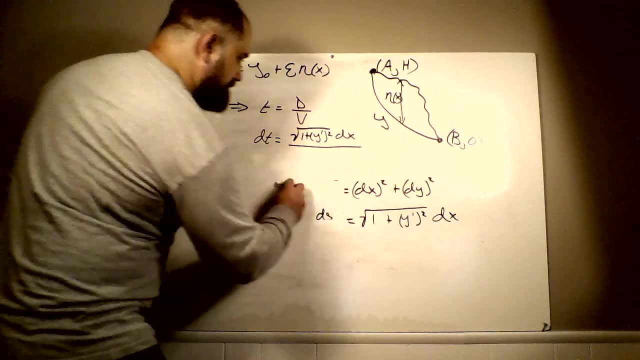 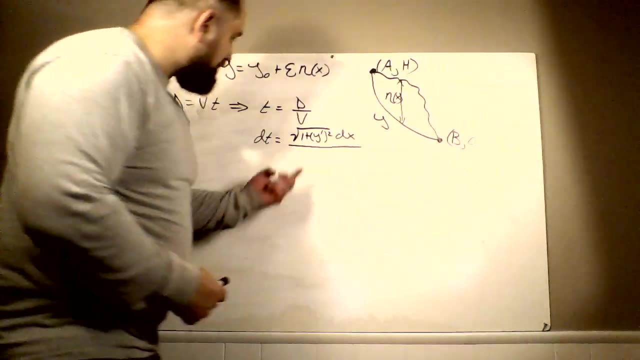 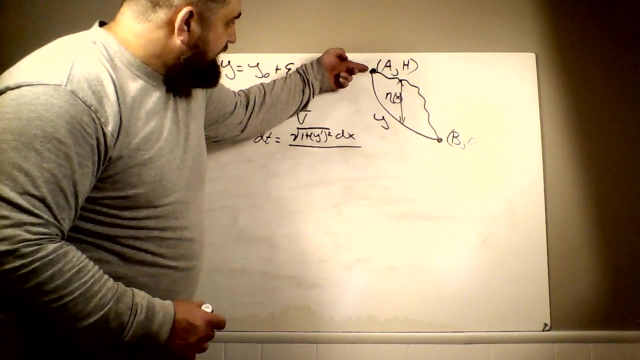 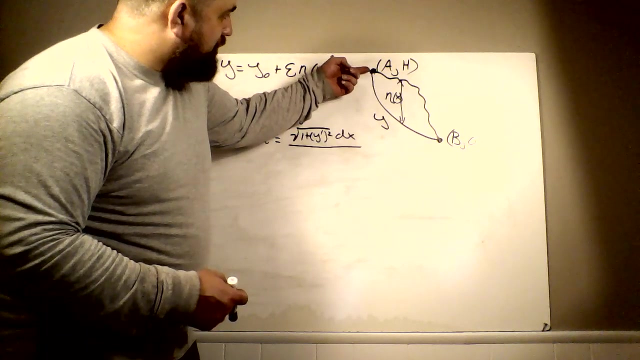 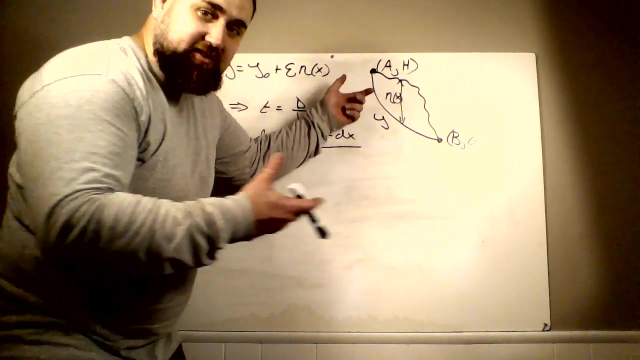 We multiply the distance between two angles and then we simplify the distance between the two angles. So the distance between the two angles it's negative or negative. and then we multiply the kinetic energy. As we drop it slowly gets converted into kinetic energy. So to write: 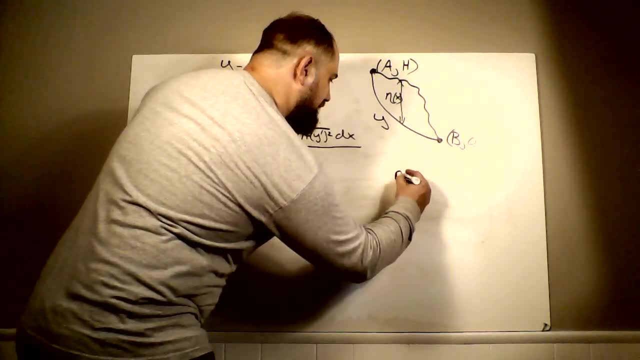 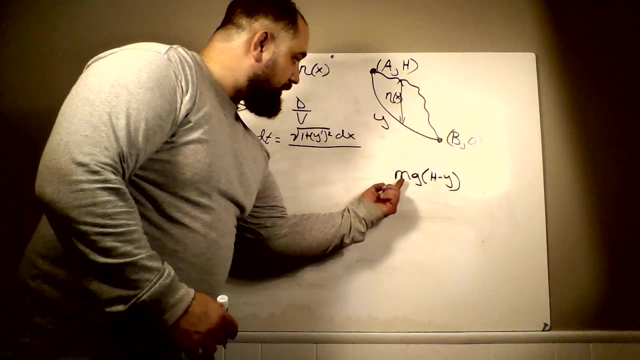 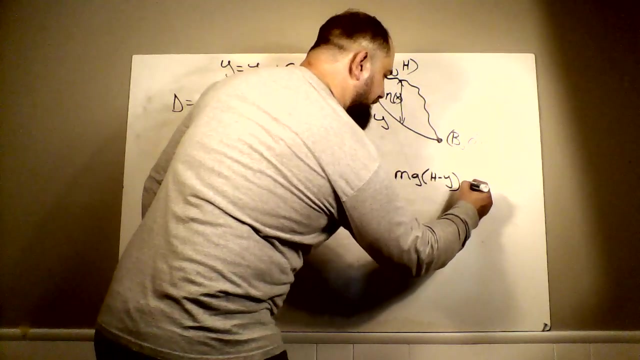 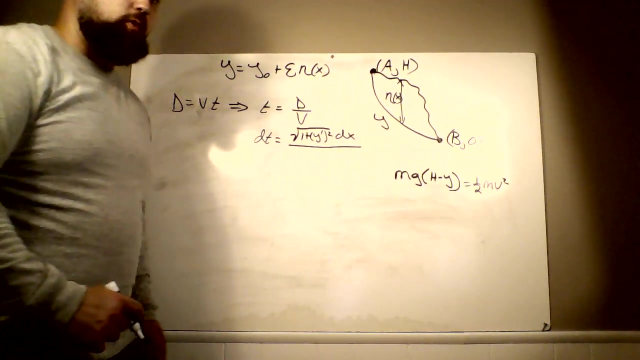 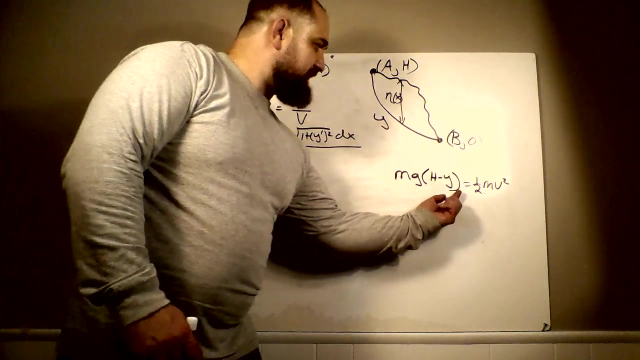 that mathematically we would say, our change in potential, our mg change in height- that's our change in potential- is equal to our kinetic One half mv squared. I think that's coming up, I can't tell if the light's blocking it. So our change in potential is equal to our. 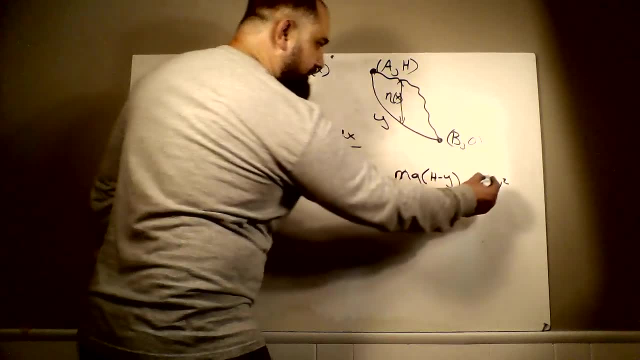 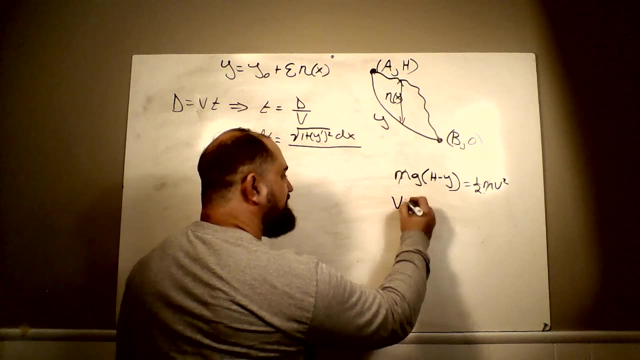 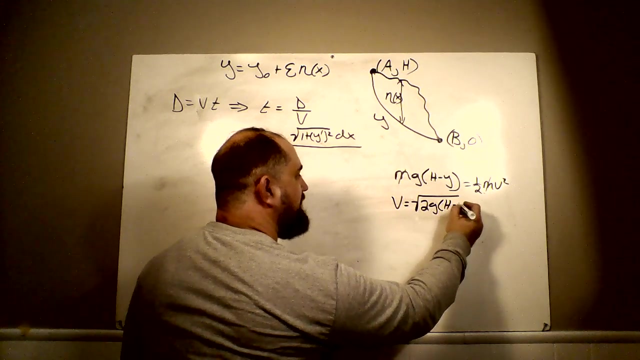 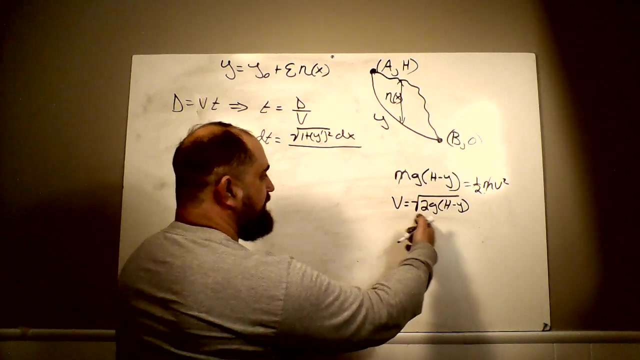 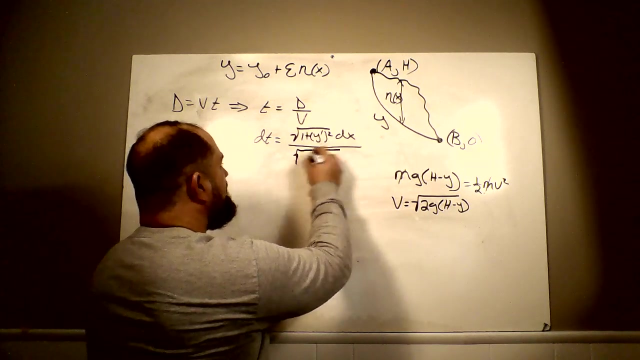 kinetic, The masses cancel out. And so if we solve for v, we get velocity. The velocity is equal to the square root of 2g times h minus y. So now we're going to take this and plug it in here for v. So we get the square root of 2g times h minus y. 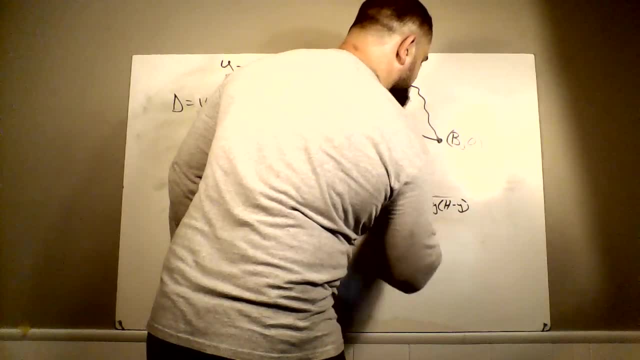 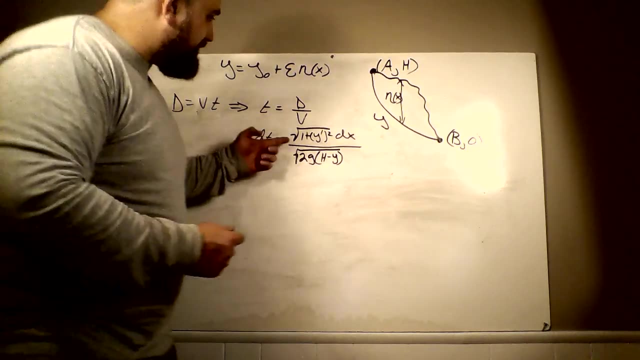 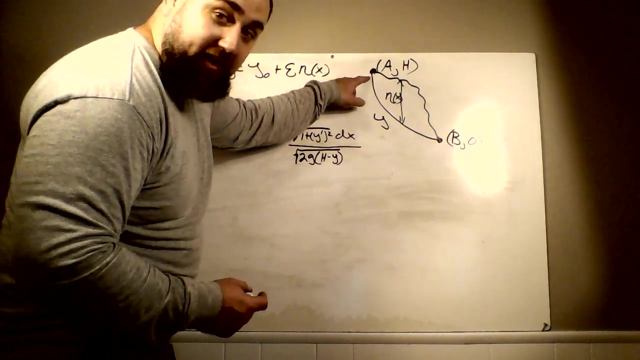 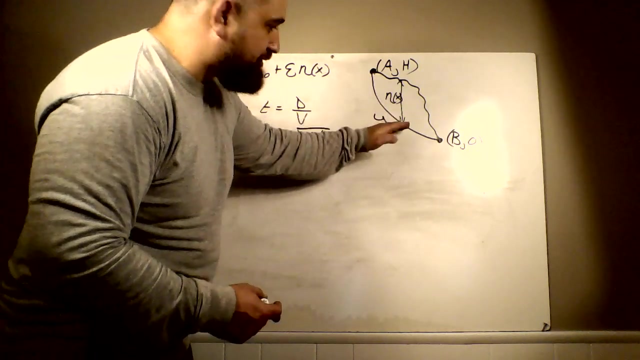 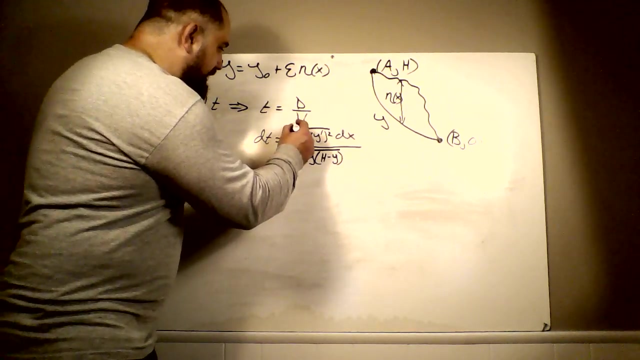 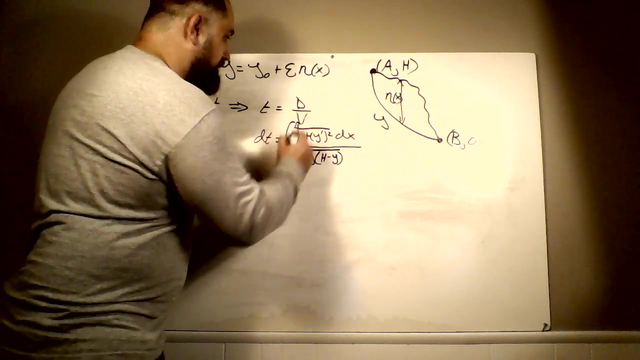 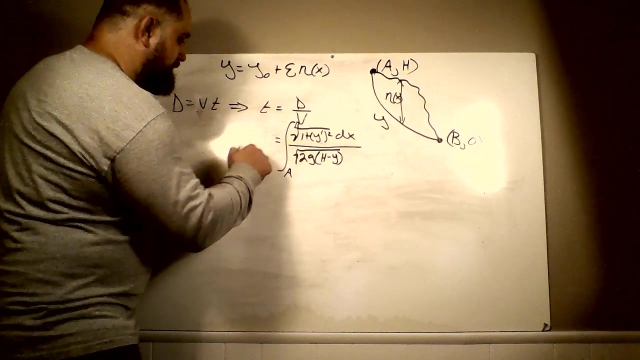 Okay, so this just tells us what the differential time would be for a differential arc length. So we need to integrate over all those arc lengths to get the total time. Okay, so Now, if we integrate from b to a, we're going to get our total time. 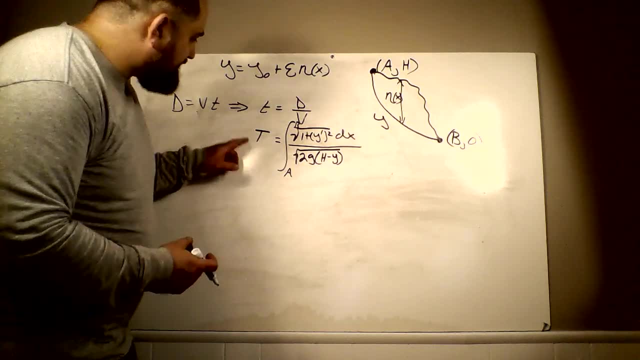 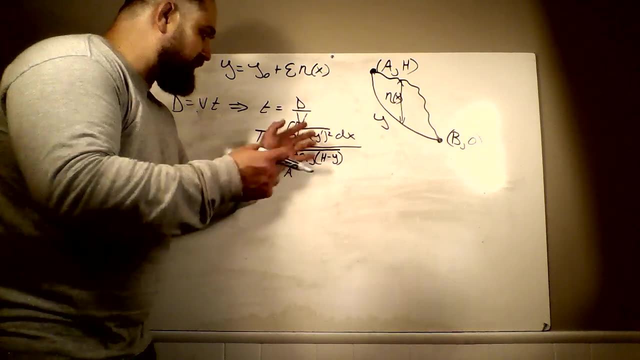 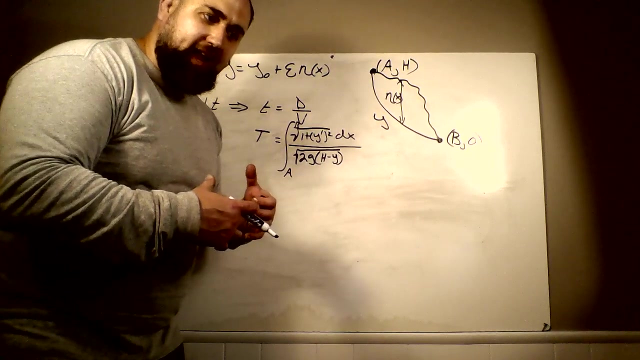 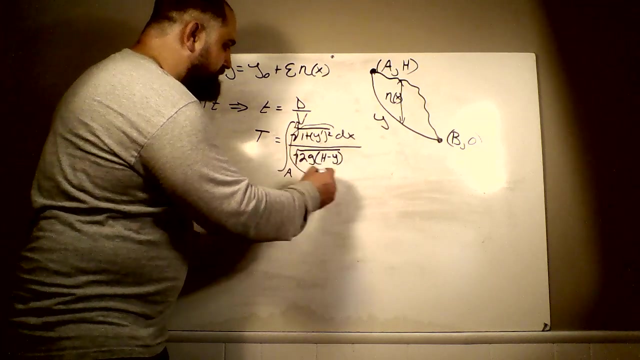 Okay, so this is true no matter what function y we put in there, Like y is equal to x squared. However, we want to apply the process of calculus of variations. We want to apply it to this to determine what y should be, to minimize time. So it's a little bit different concept, Like. 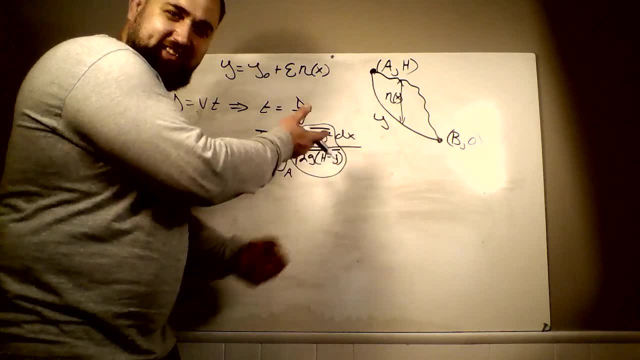 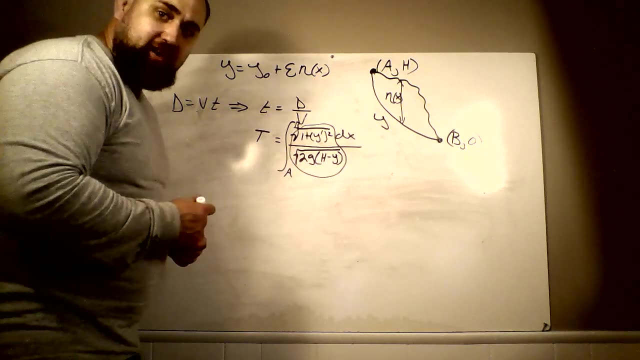 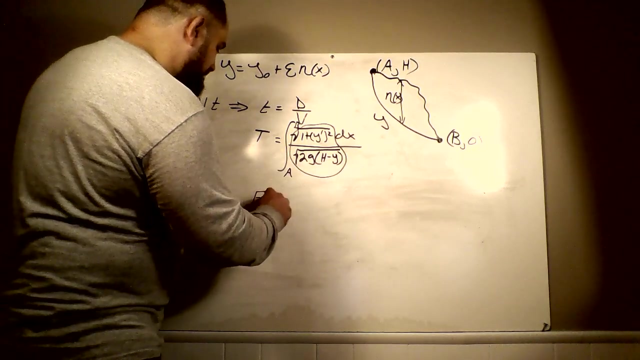 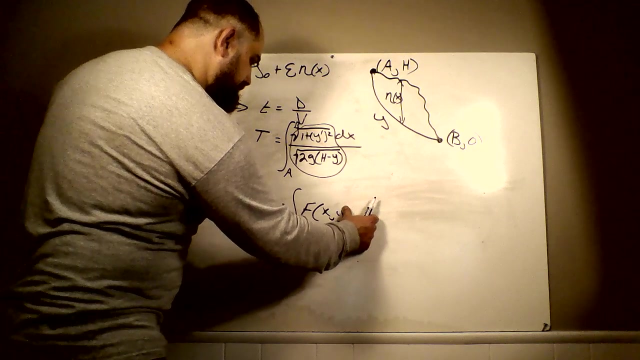 we're trying to derive what the function should be inside the integrand. But this is going to be the general structure. Where you have sooner quantity that you're trying to minimize, You have an integrand. It's usually written like this: So sum quantity e is equal to a function of x, y and y prime. We don't directly or explicitly 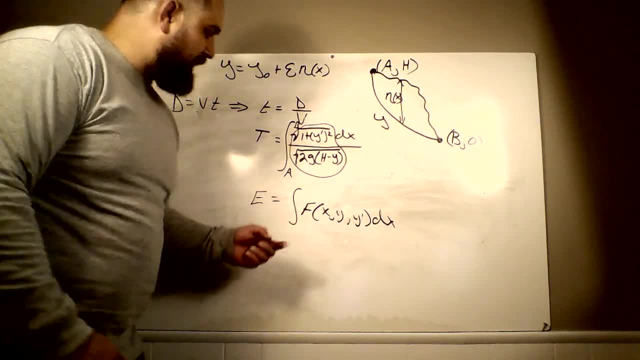 have x in here, but we have y right here and we have one function- y- in here. So what I'm trying to remember is we had x growing in here and x went off here, But also we had a function and y went right out of here. 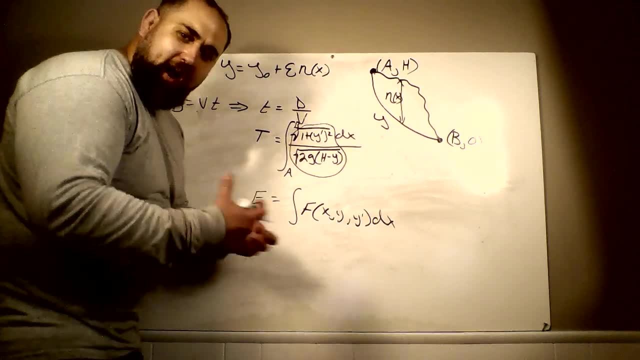 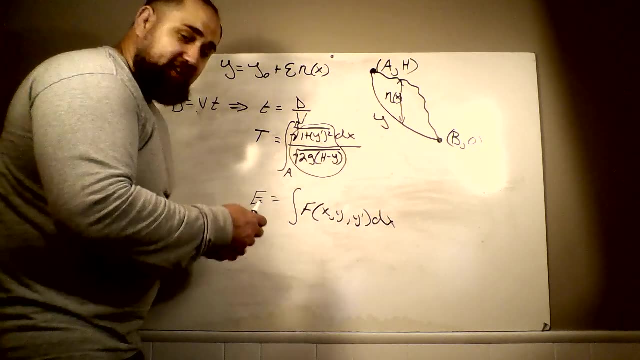 And we have y prime right there, And so we're going to derive the Euler-Lagrange equation, which is what we're going to apply to the integrands, And it's going to give us a differential equation that we solve to figure out what y needs to be. 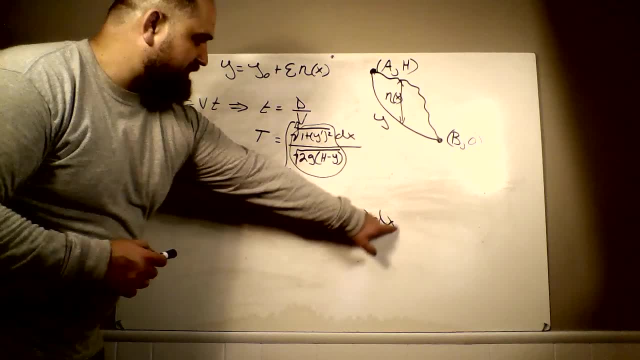 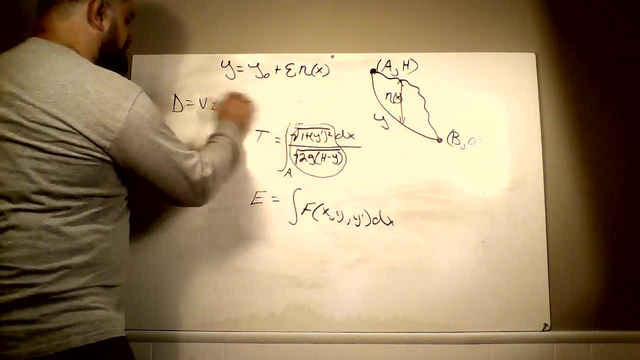 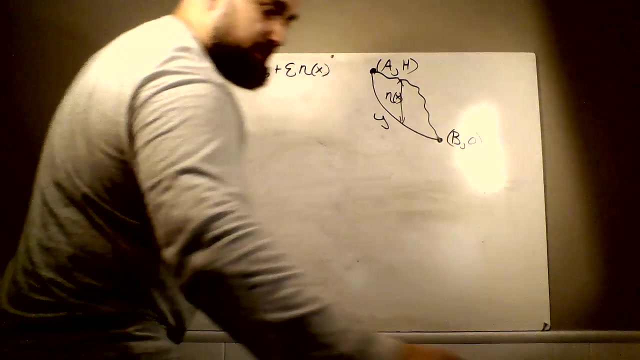 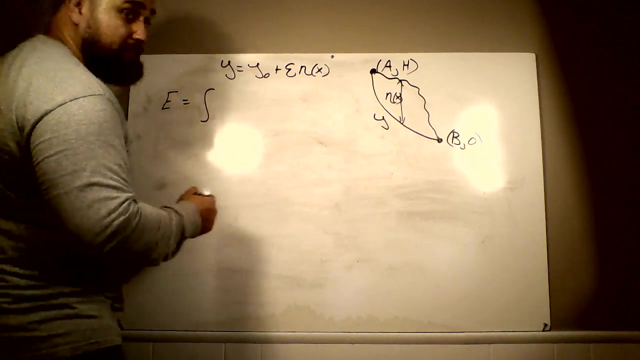 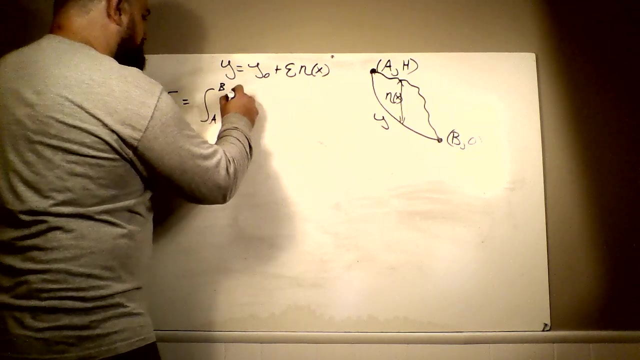 Okay, So we're going to use this in the next step here. Okay, so we have. E is equal to the integral. I'm going to put boundaries on it, So I'm going to go from B to A of f, of x, y, y, prime dx. 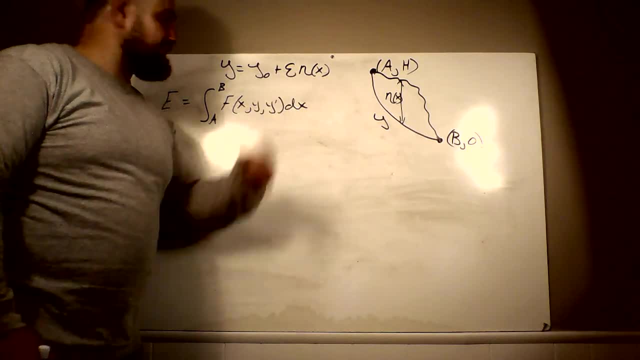 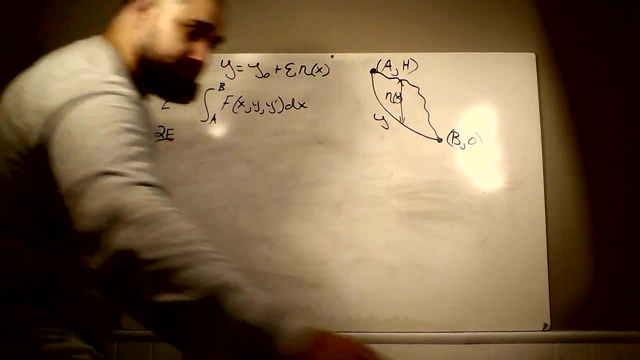 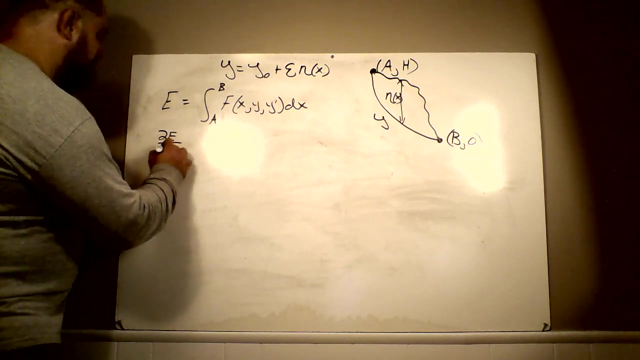 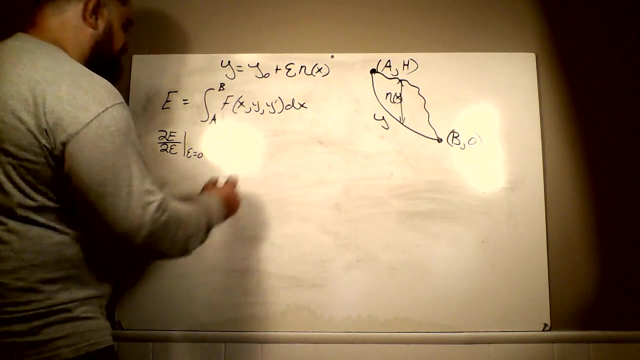 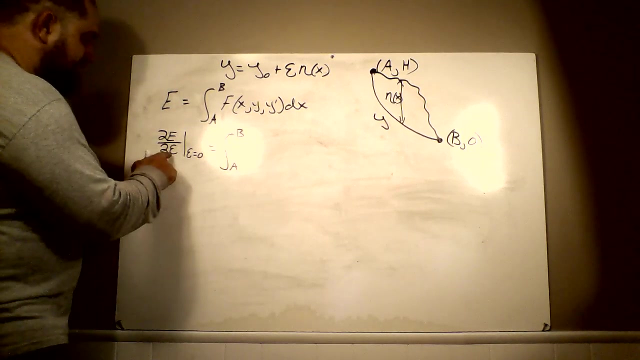 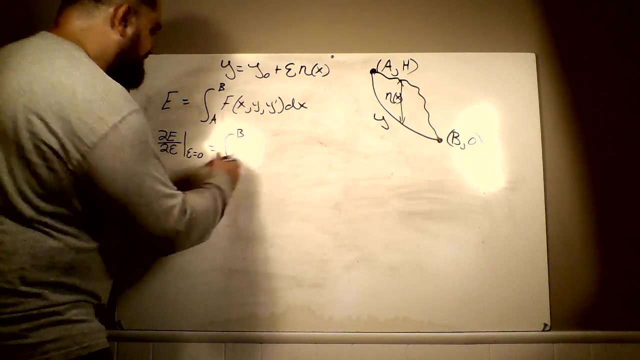 And I'm going to differentiate this with respect to epsilon. So I have partial E over partial epsilon. evaluated at, epsilon is equal to zero, is equal to A- B, Because epsilon is not dependent on x and vice versa. I can put the differential sign inside the integral. 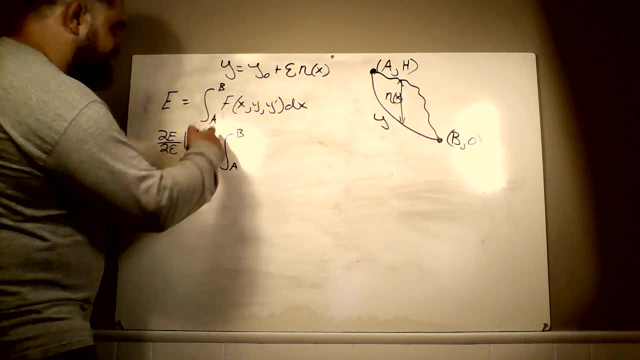 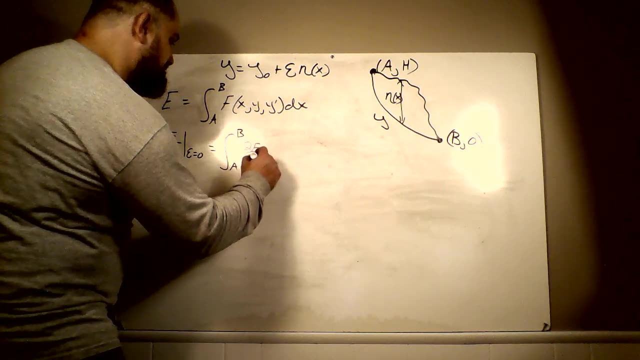 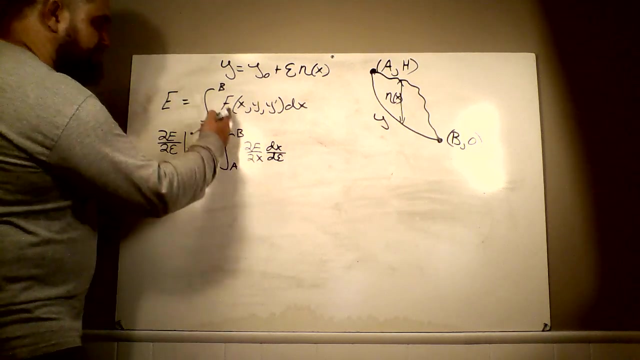 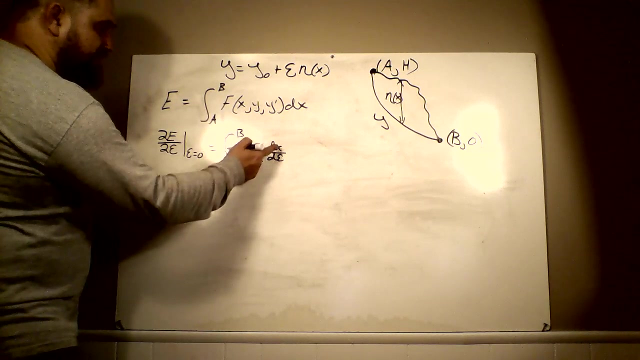 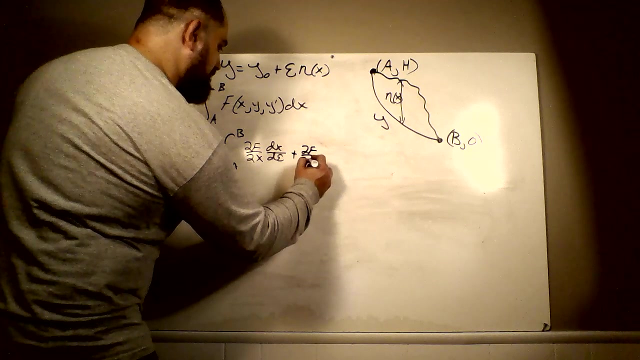 And I have to first differentiate f with respect to x. So I have partial f over partial x, dx over d epsilon. So I've differentiated f with respect to x, that applied the chain rule, and differentiated x with respect to epsilon, Plus partial f over partial y, dy over d epsilon. 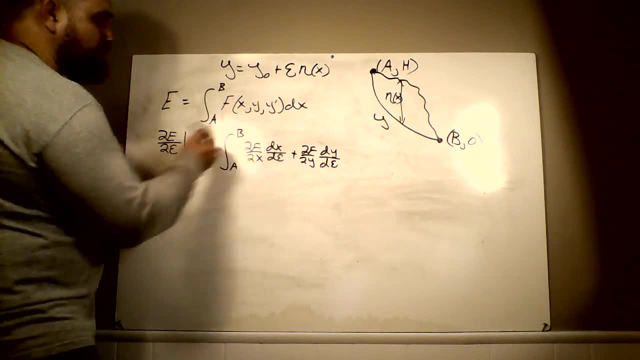 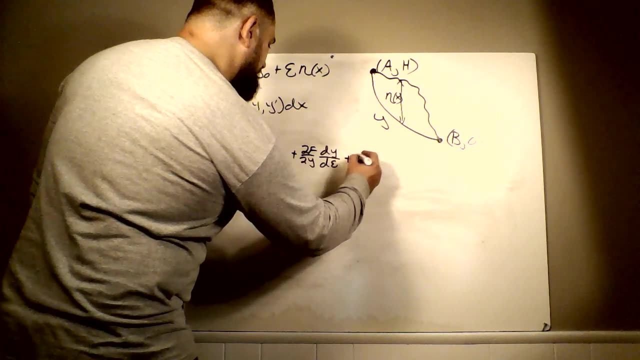 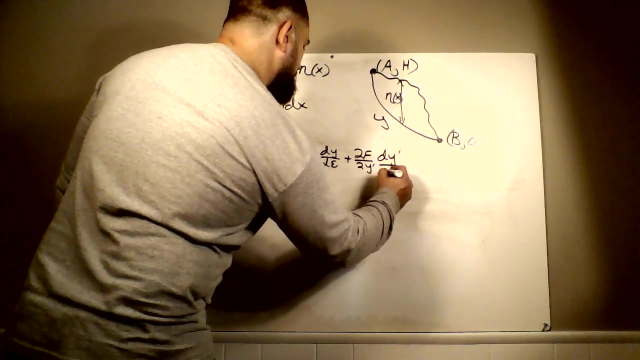 So I've done the same thing: Partial f with respect to y. And then the chain rule says I have to differentiate y with respect to epsilon Plus partial f over partial y, prime, dy prime over d epsilon. Now we close her off here. 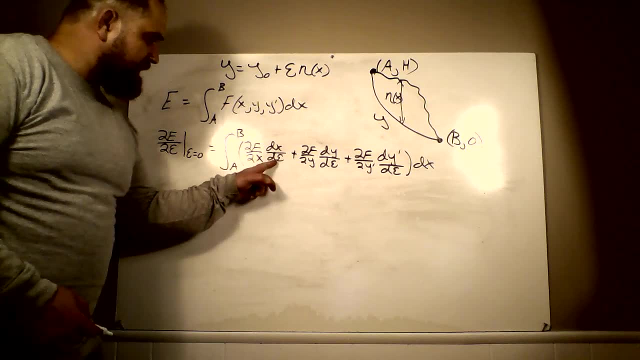 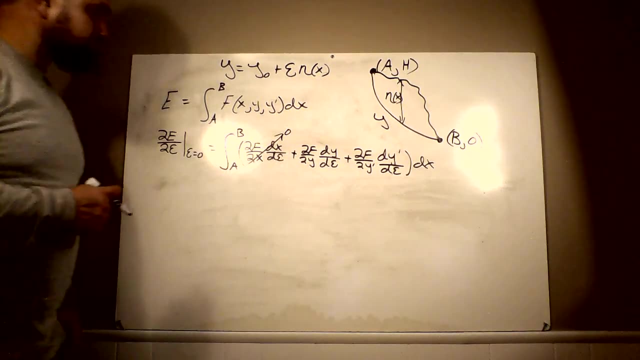 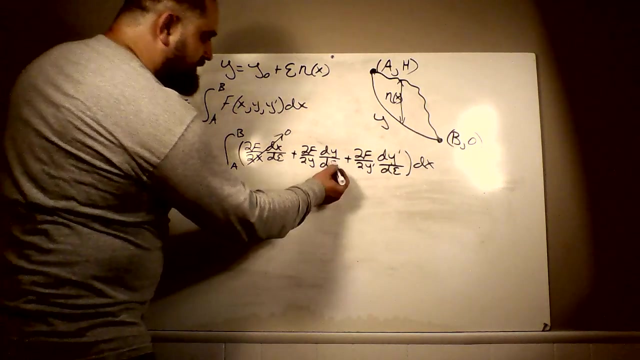 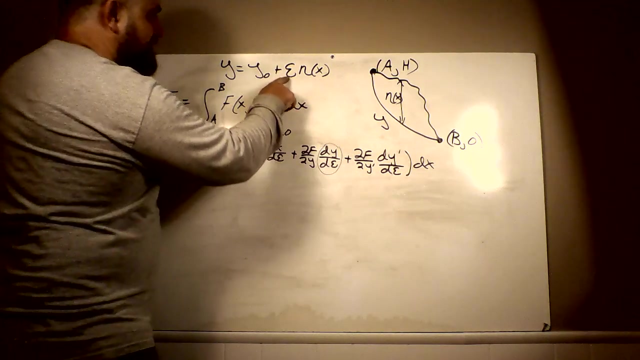 Here, x is not dependent on epsilon, and vice versa, So the derivative is just going to go to zero. Epsilon is not a function of x dy over d- epsilon. If I differentiate this with respect to epsilon, I just get eta. 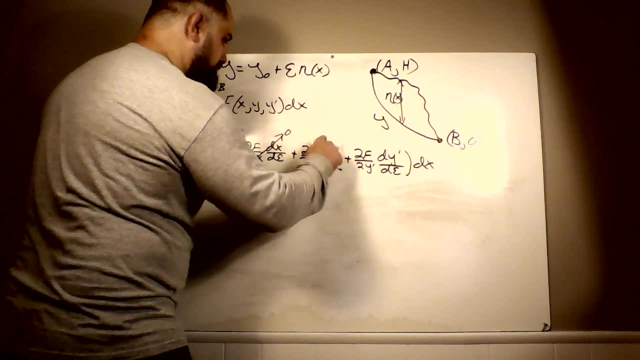 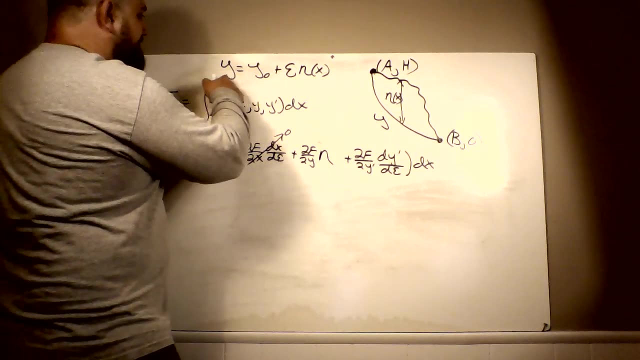 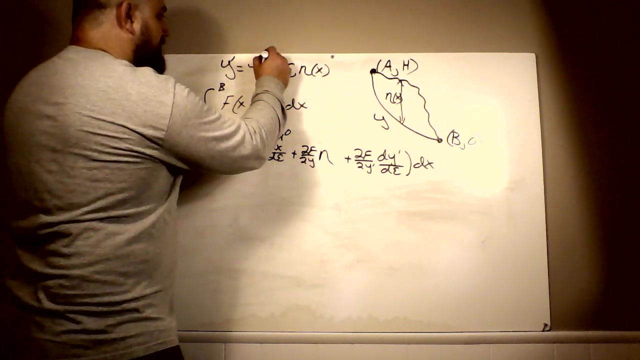 So stands for radical x, d over x. So this term here is eta. If I differentiate this with respect to x, I get y prime equals y0 prime plus epsilon eta prime. If I differentiate this with respect to x, I get y prime equals y naught prime plus epsilon eta prime. 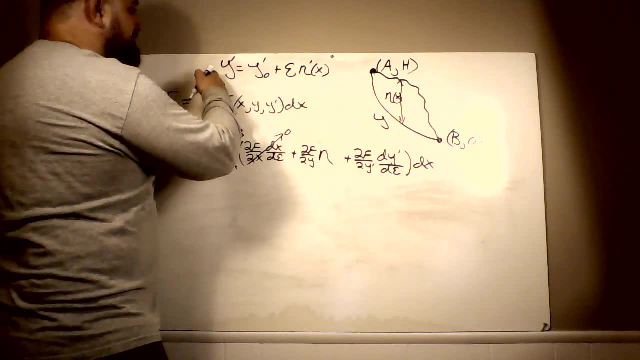 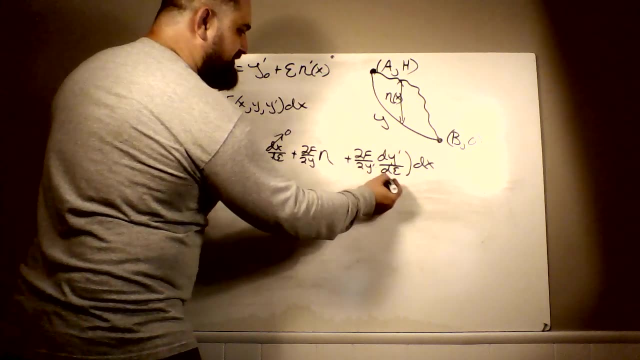 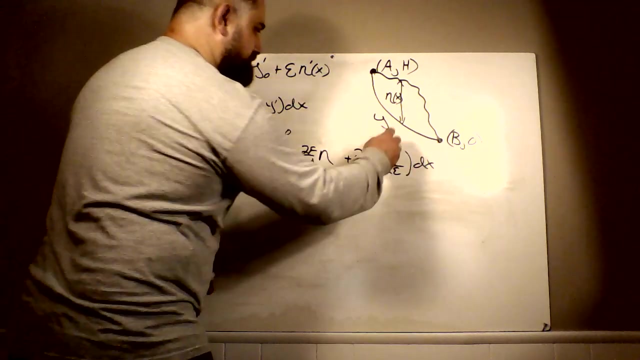 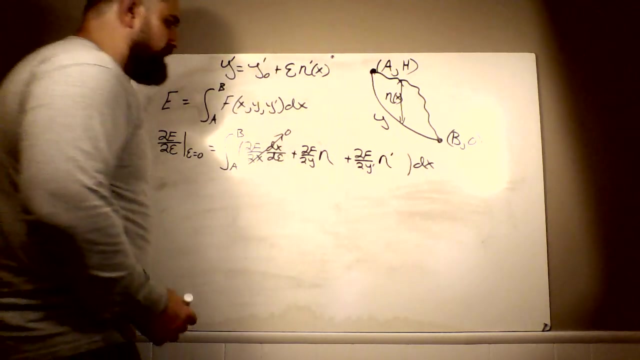 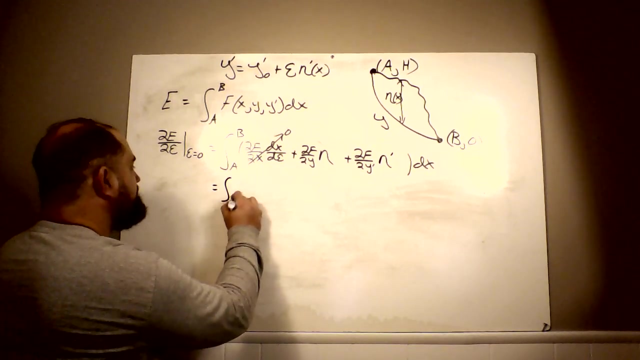 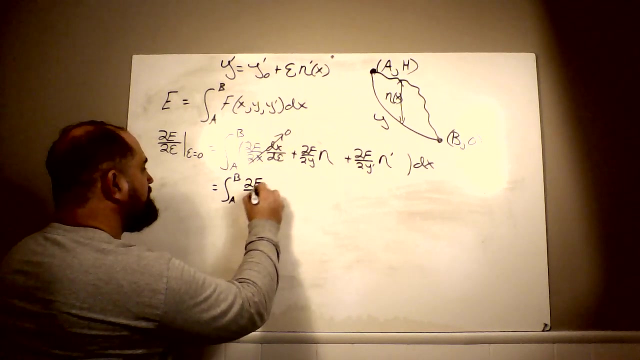 Epsilon plus epsilon Epsilonтив. If I differentiate this with respect to epsilon, I get eta prime. So this term is just eta prime. So now we're going to do a bit of integration by parts. We're going to keep this first term inside the integral. 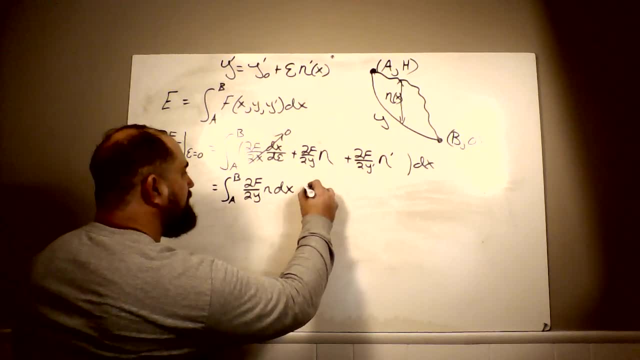 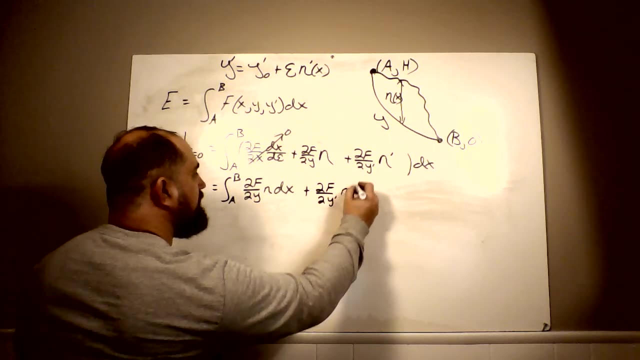 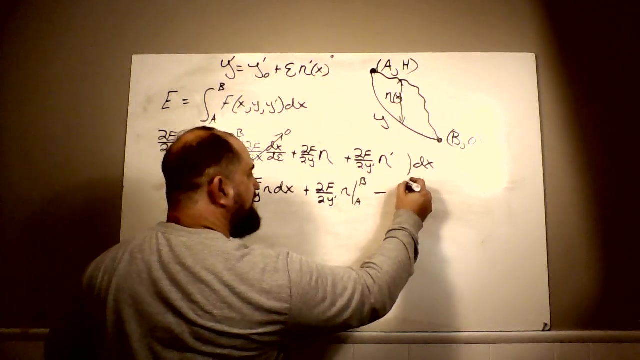 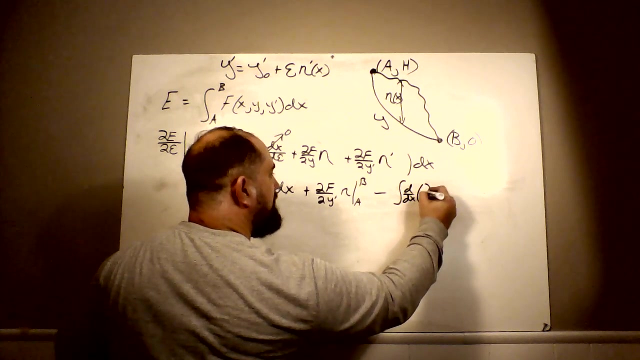 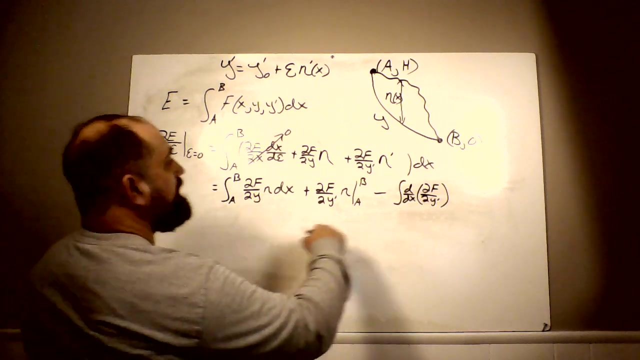 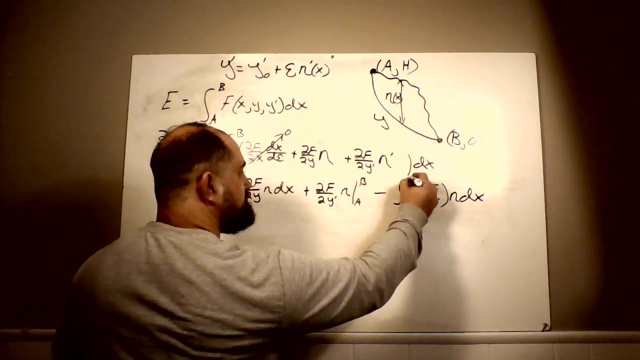 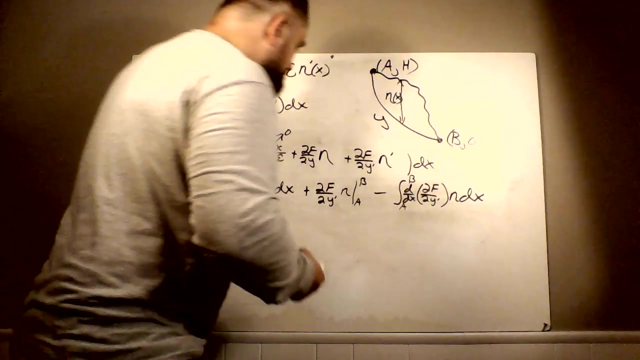 And we're going to integrate this part by parts, Plus, this times, the integral of this, Minus the integral of the derivative of this Times, the integral of this And this, which is just eta. Okay, Now look at this here. 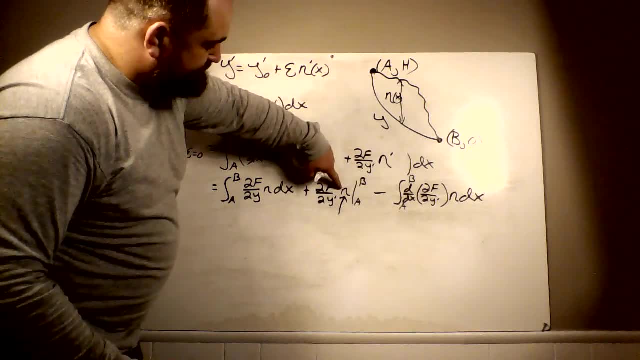 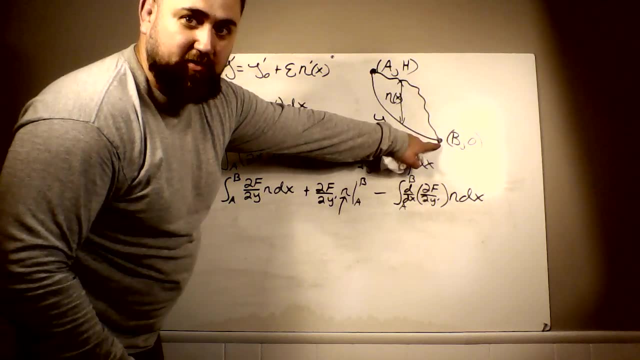 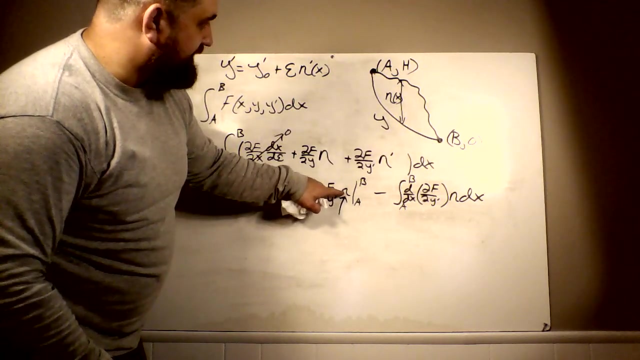 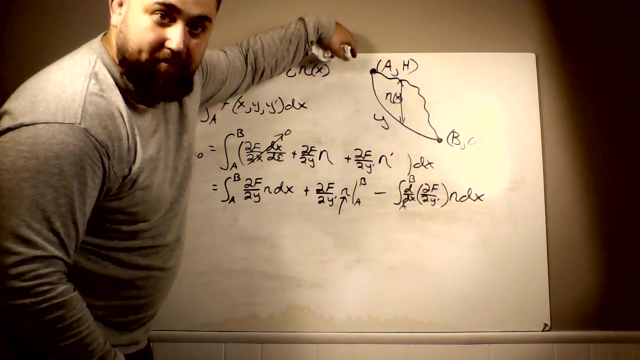 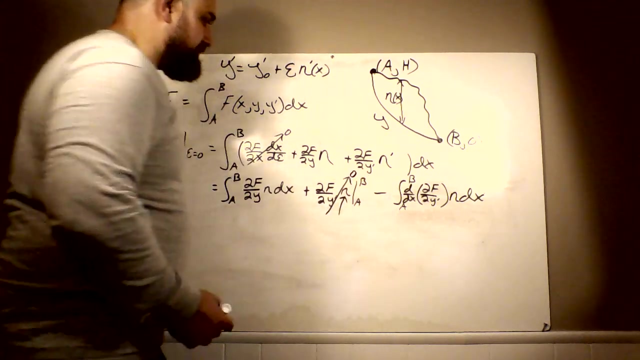 When you put b into eta, eta is zero and x is equal to b. Likewise, when you put a into eta, eta is zero, at x is equal to a. So there's no variation at the endpoints. So this term goes to zero. 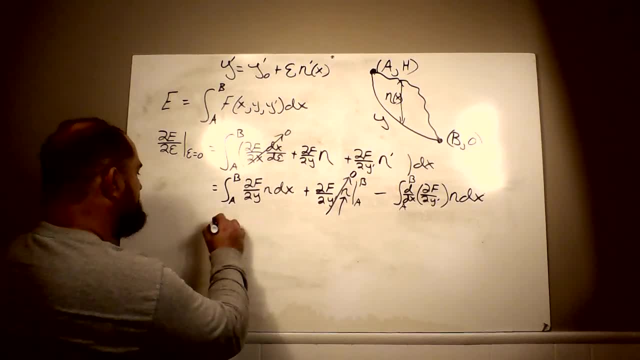 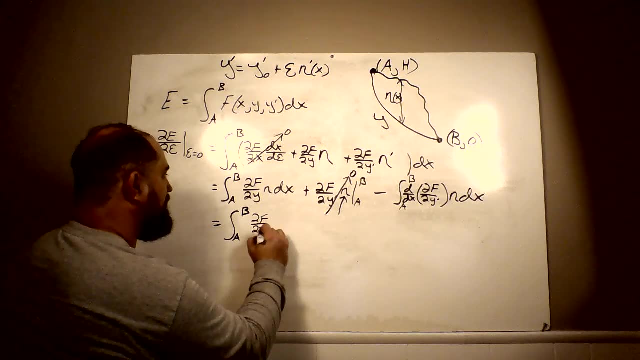 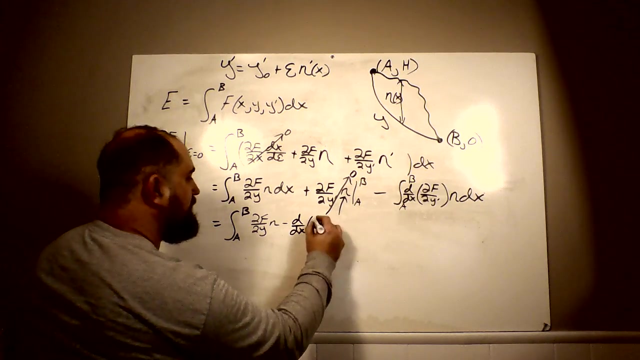 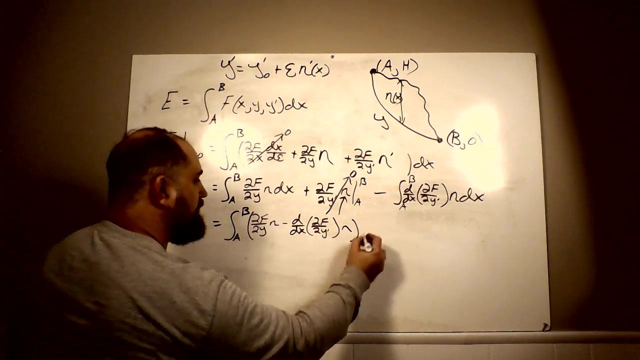 So now we can combine the two terms. So again we're going to do a bit of integration by parts. We get partial f over partial y, eta minus d over dx, partial f over partial y, prime eta dx, And just combine these two integrals into one. 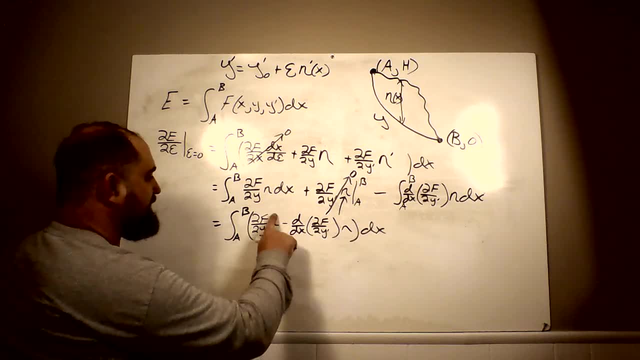 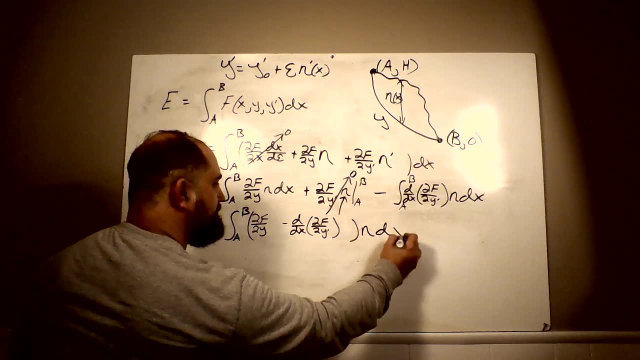 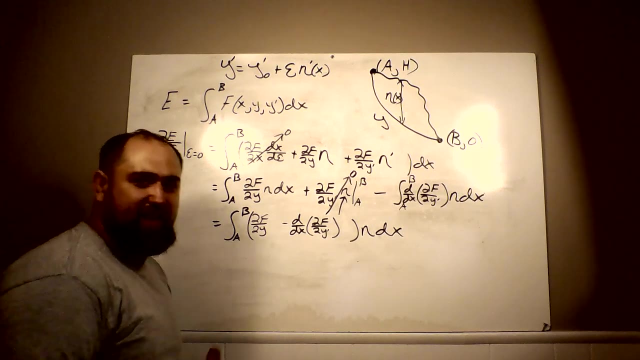 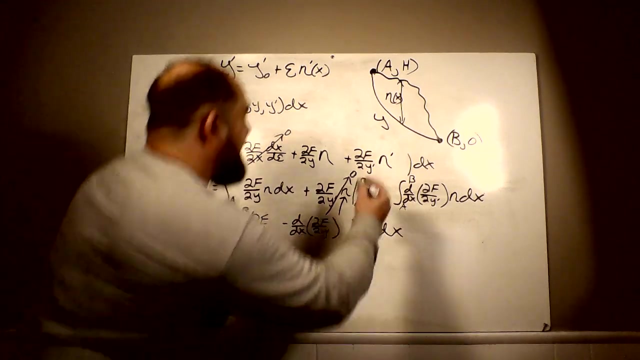 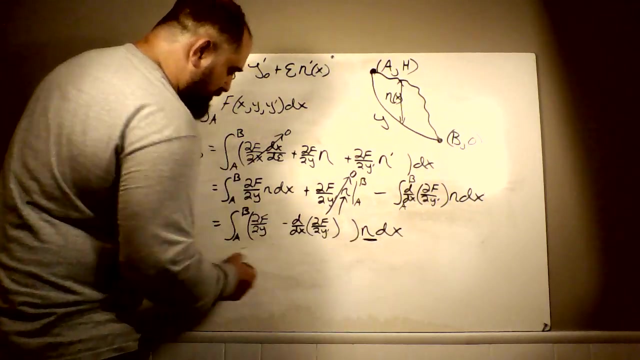 They both have eta in them, So I'm going to factor out eta. So this is some quantity like time, distance, energy, velocity that we're trying to minimize, And eta has no bounds, And so the only way to guarantee that this integral is minimized, 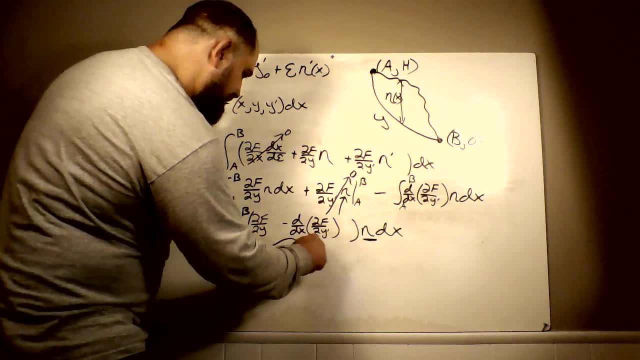 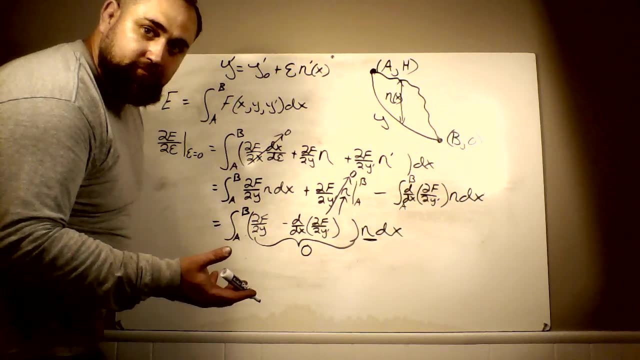 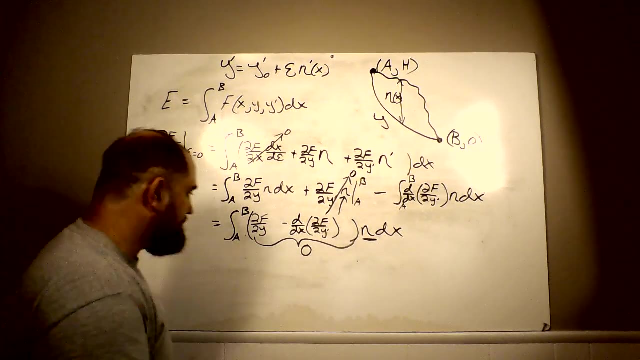 is to do a little bit of integration, And then the other way to do it is to say that what's inside the parentheses is zero. So this is what's called the Euler-Lagrange equation. They typically write it as partial f over partial y, minus d over dx. 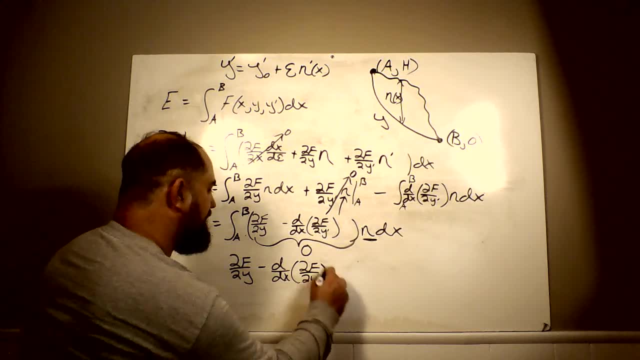 partial f over partial y prime is equal to eta. And we've got this in the state. And so now we know that e to e to e to f we've got to write as partial f over partial y, minus d over dx. partial f over partial y prime is equal to eta. 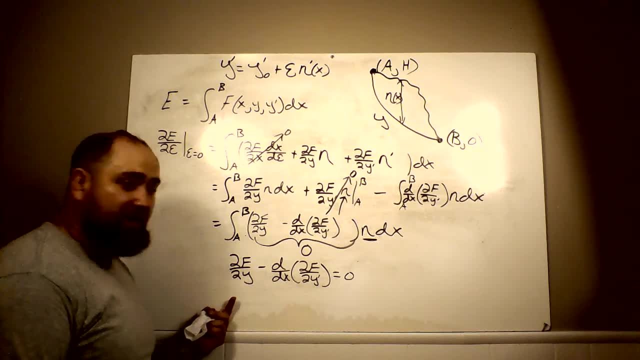 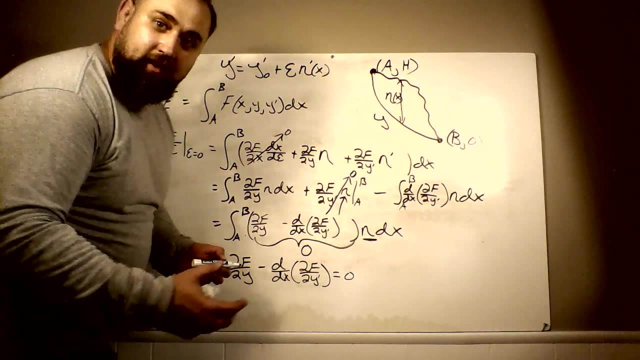 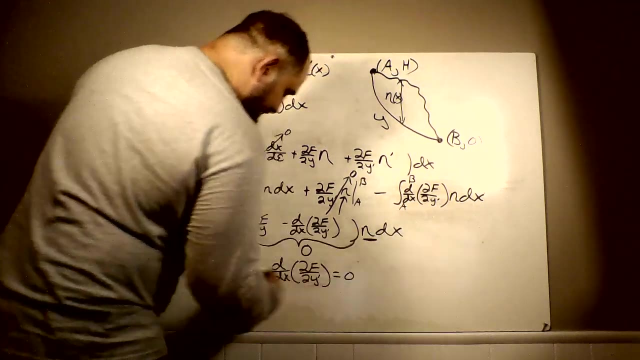 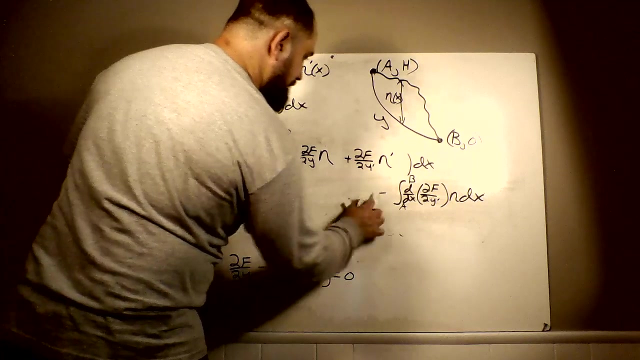 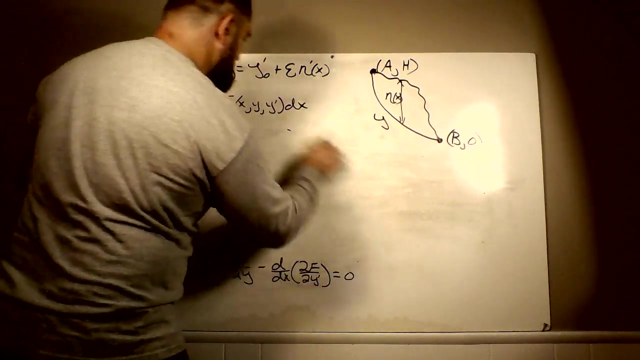 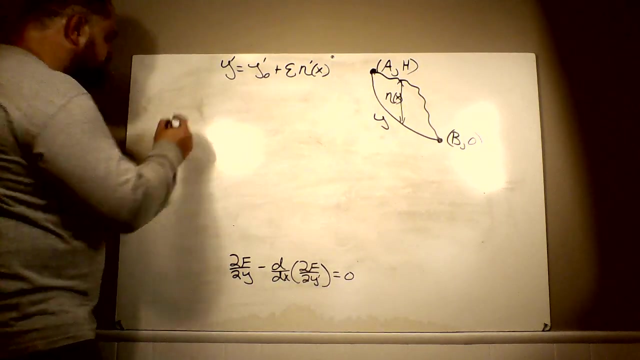 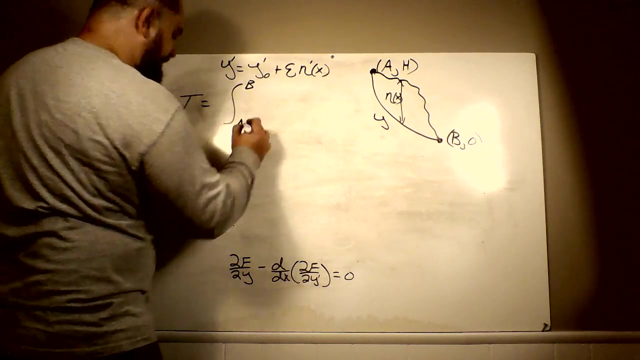 zero. This is the Euler Lagrange equation. We're not going to solve the problem that we did before, but we're going to just kind of look at it real quick. so we know what to do with this. okay, so we had: T is equal to the integral from b to a of the square root.